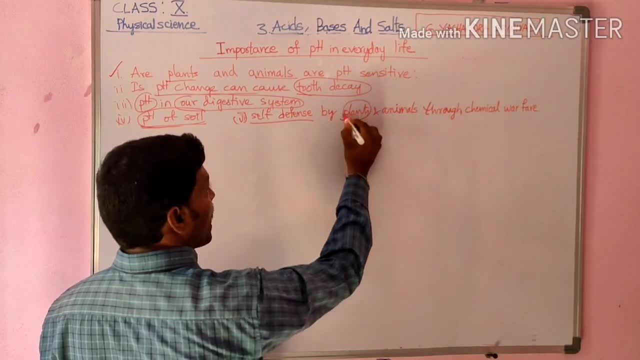 Next, self-defense by plants and animals through chemical warfare. 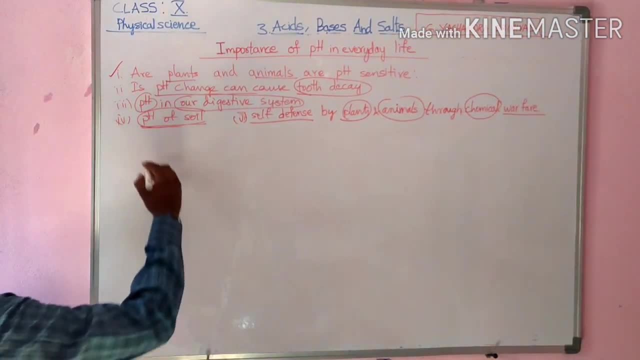 Right, so that is we are going to learn. In the first one, plants and animals are pH sensitive. 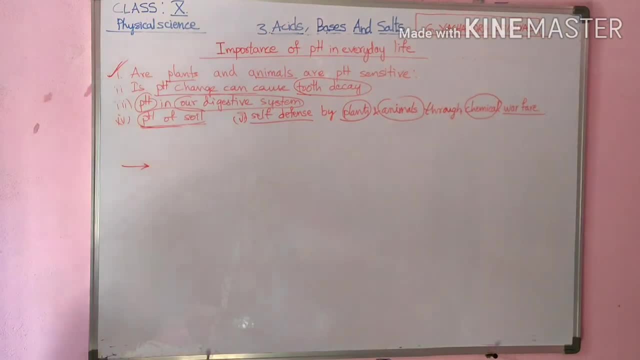 In living things, so many chemical activities take place. So many metabolic activities occur. And all the chemical activities, all the metabolic activities occurs at a particular pH level. So, the change in pH will affect the metabolic activity. For example, if you take digestion. Digestion, right. 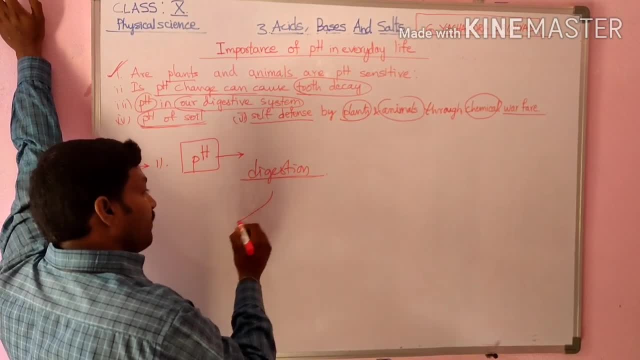 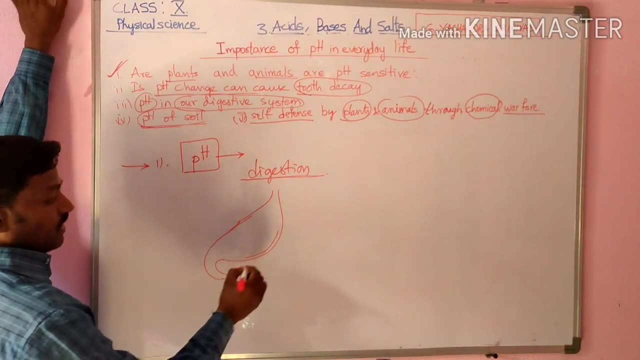 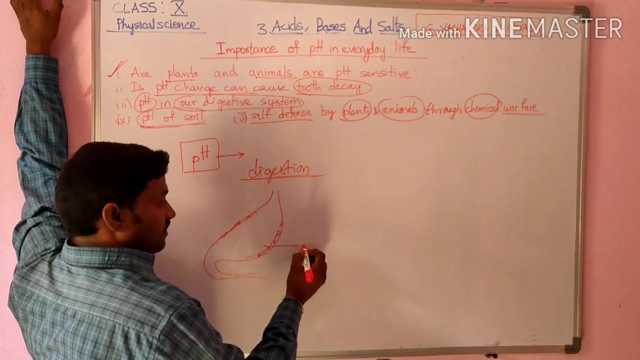 So, in this, if you see in the stomach, in the stomach, right, there is a digestive juice called a gastric juice. It secreted by the gastric glands in the stomach. And that gastric gland secretes gastric juice and that contains hydrochloric acid. Hydrochloric acid. Right. 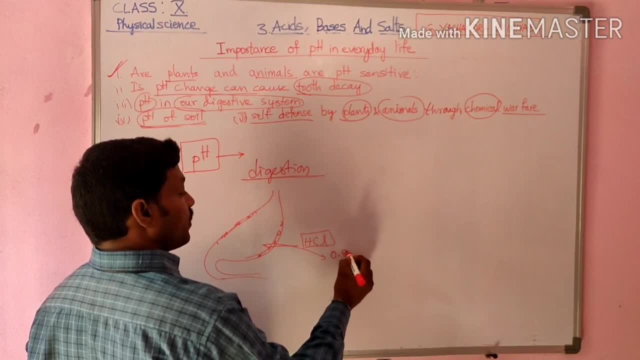 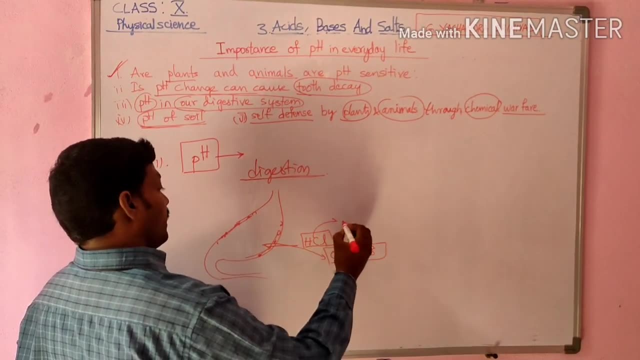 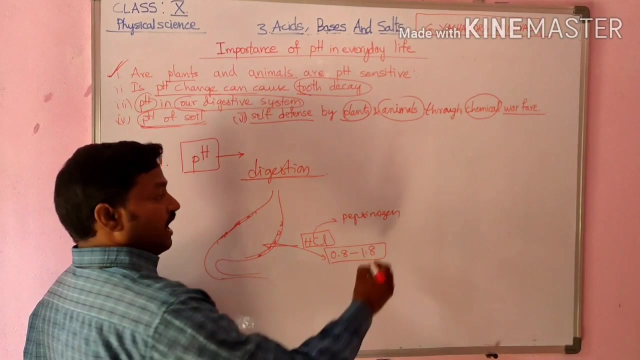 And the pH of this acid is about 0.8 to 1.8. Right. So, at this pH, what happens? What happens? The pepsinogen. Pepsinogen. Right. It is an enzyme, but it is in active form. In active form. Right. 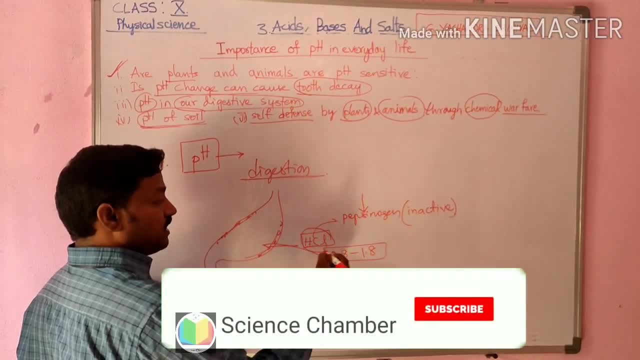 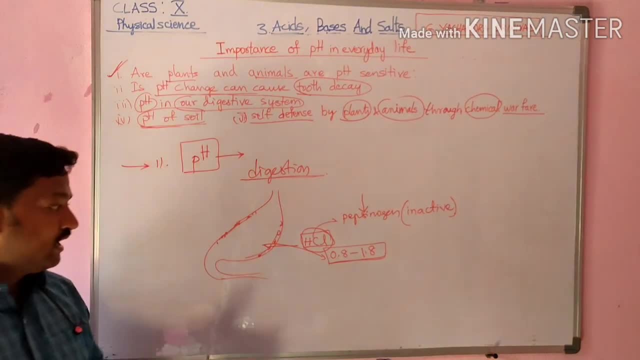 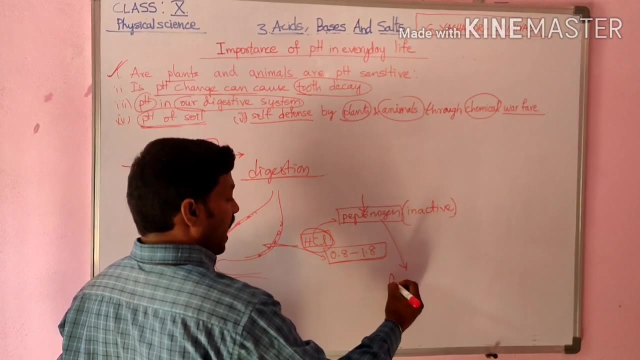 So, this will be get activated. By the acidic medium due to HCL. What is that pH? 0.8 to 1.8. At this pH, then what happens? This pepsinogen will be converted into or becomes active. Active pepsin. 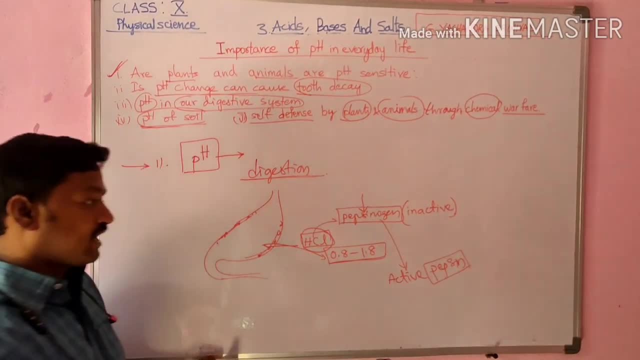 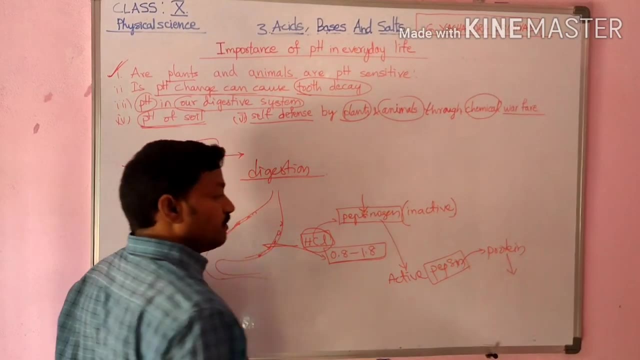 Pepsinogen becomes pepsin, which is an active form. Then, this pepsin acts on proteins and convert them into simple proteins. And convert them into simple forms called peptones. 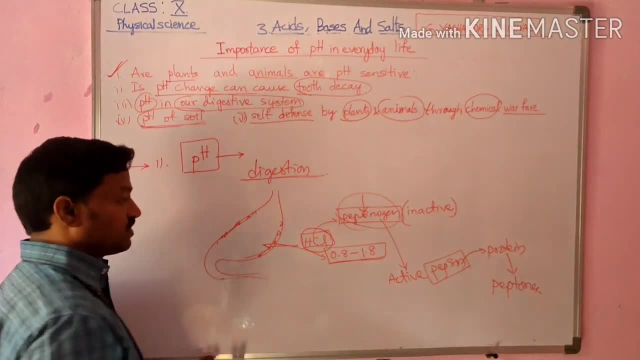 So, that means this action or this reaction will take place in acidic medium. 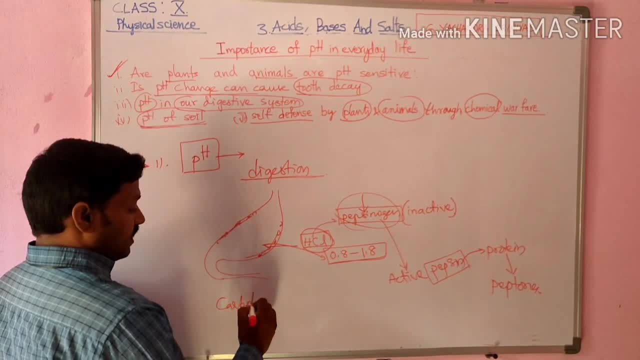 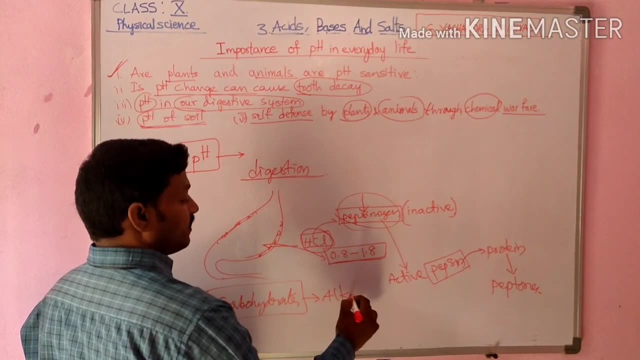 Whereas, the digestion of carbohydrates. Digestion of carbohydrates. For the digestion of carbohydrates, requires alkaline medium. 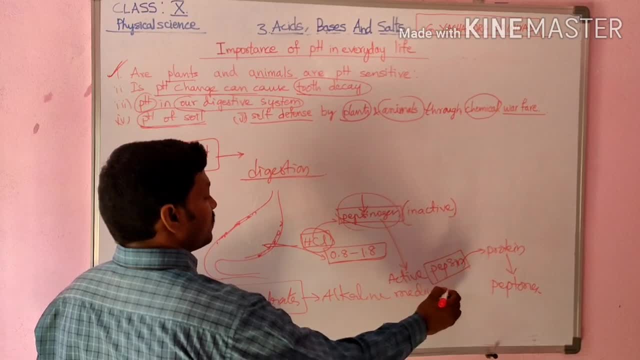 Alkaline medium. So, that means all the activities in the liver. Okay. 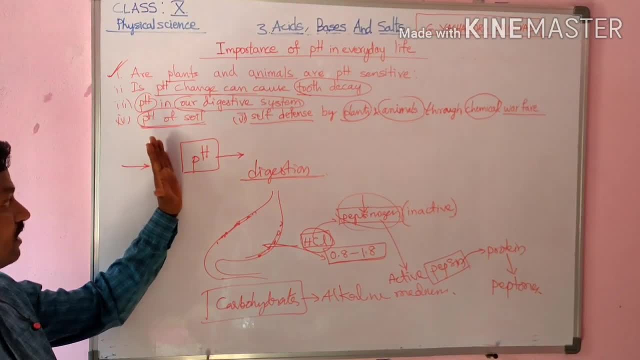 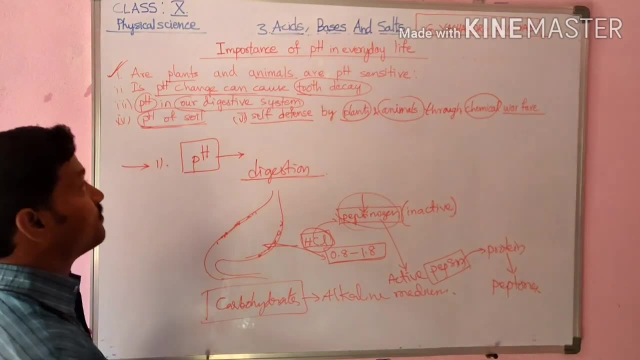 All the activities in the living bodies will occur at a particular pH. If there is a change in the pH, then the survival of the organisms becomes difficult. Survival of the organisms becomes difficult. 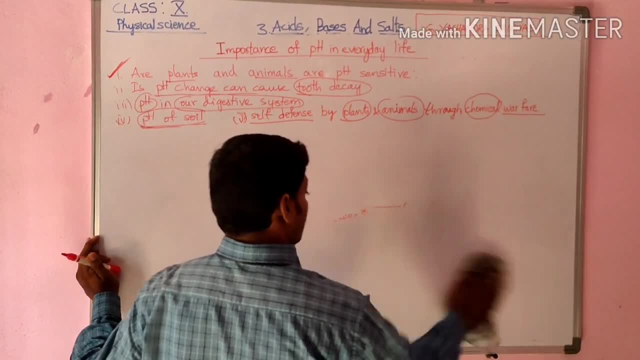 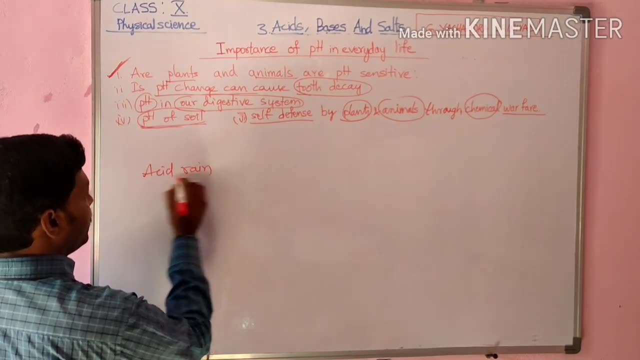 Let us suppose here, let us take acid rain. What is that? Acid rain. Acid rain. Acid rain. 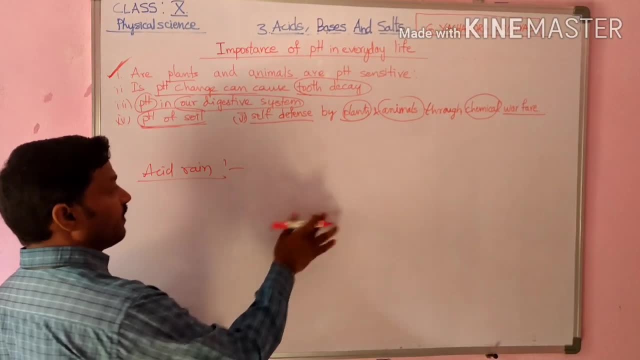 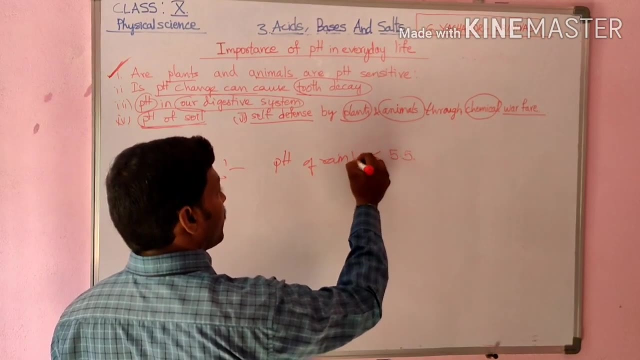 What is acid rain? Right. So, when the pH of rain. When the pH of rain is less than 5.5. 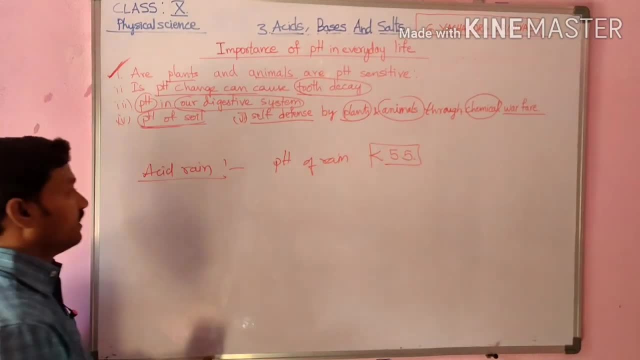 When the pH of the rain is 5.5, then that rain is called acid rain. 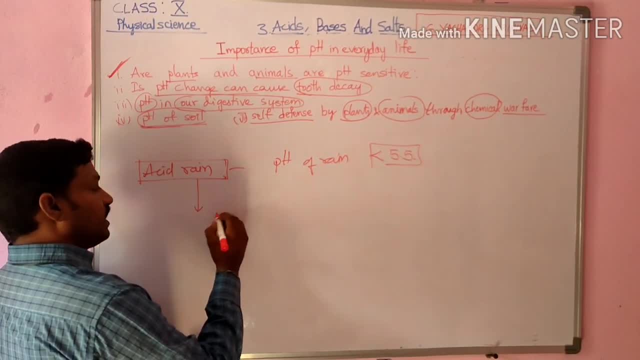 So, why is the acid rain? Right. So, in the atmosphere, when the pollutants are more, like carbon dioxide, sulfur dioxide. Right. So, next, nitrogen dioxide. 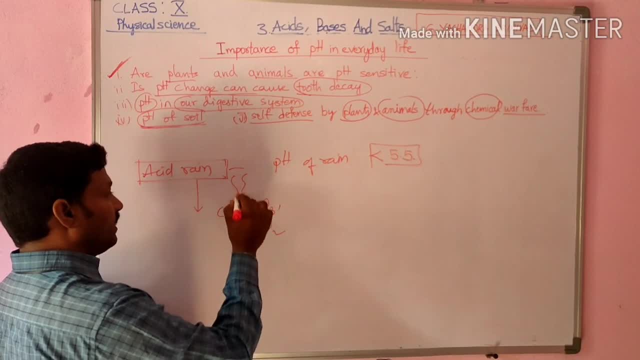 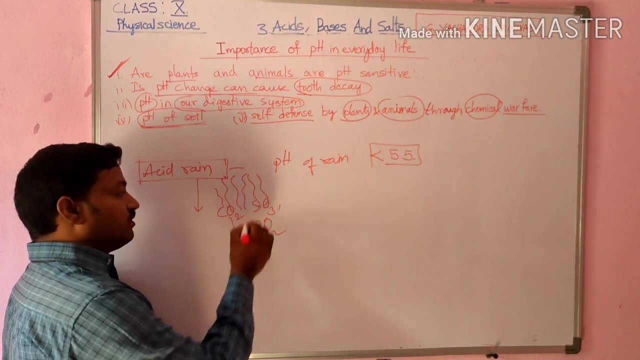 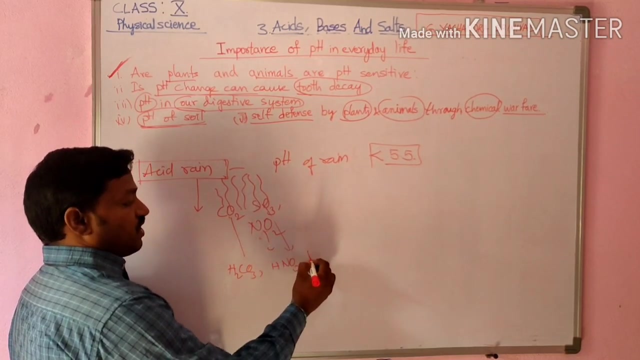 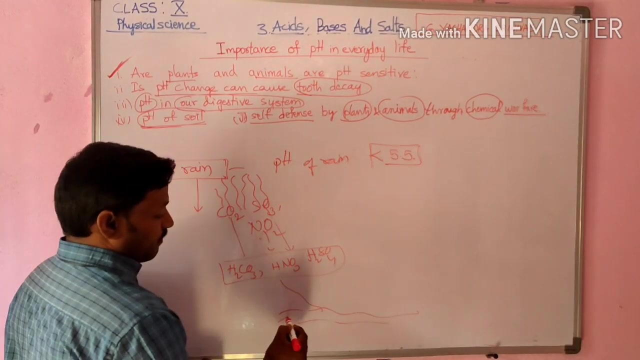 So, what happens during the raining? The water contact with these non-metal oxides, then they will give the respective acids. What are the respective acids? Carbonic acid, nitric acid, sulfuric acid. Right. When they descend to the earth's surface, then what happens? They flows on the earth and reaches the river water. Right. 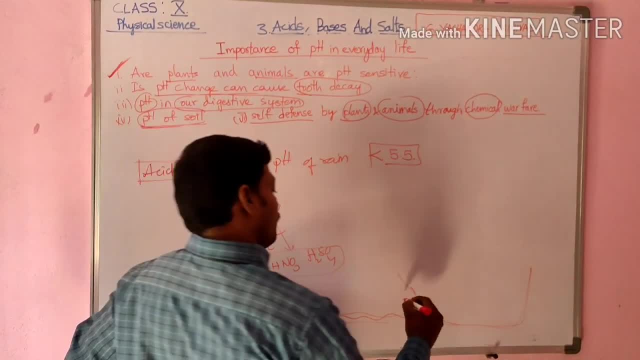 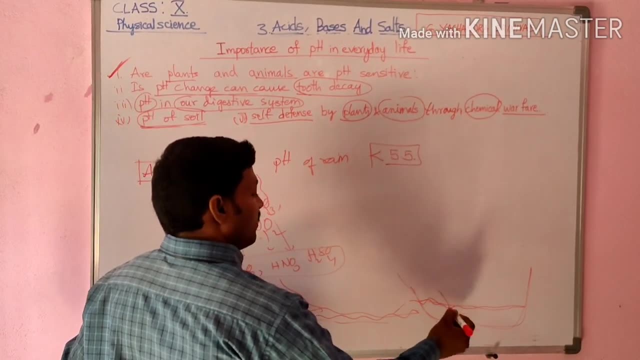 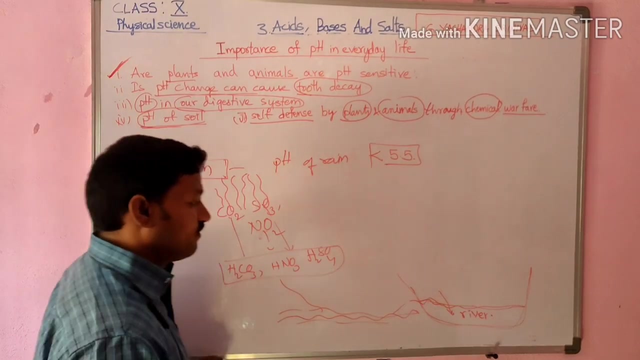 So, when this acid rain will get mixed up with the water, then this acid rain will change the pH of the river water. 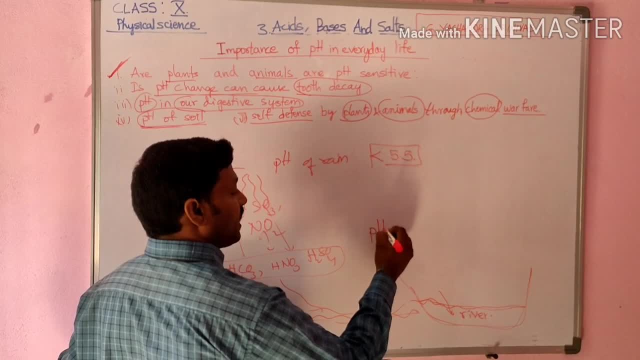 It will change the pH of the river water. So, when acid is getting mixed up with the river water, the pH will decrease. Ph decreases. When the pH decreases, what happens? Acidic carbon dioxide. 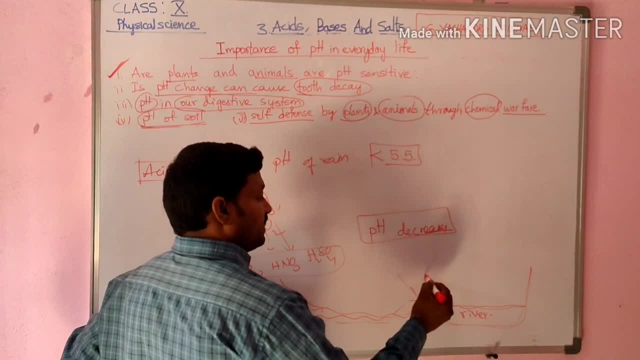 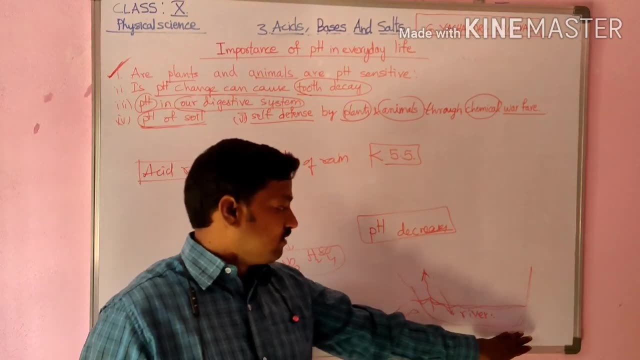 acidic character increases so when the acidic character increases then what happens the plants and animals which are living in this river water will be get affected so the change in the p-head 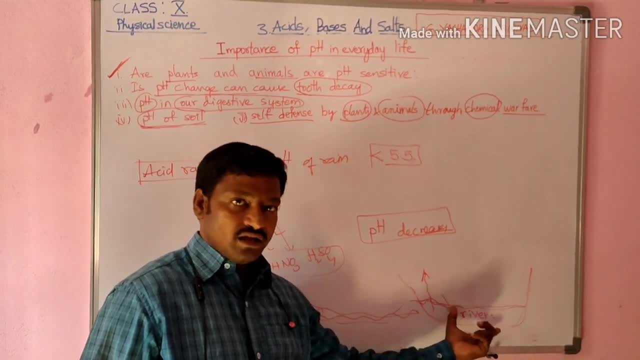 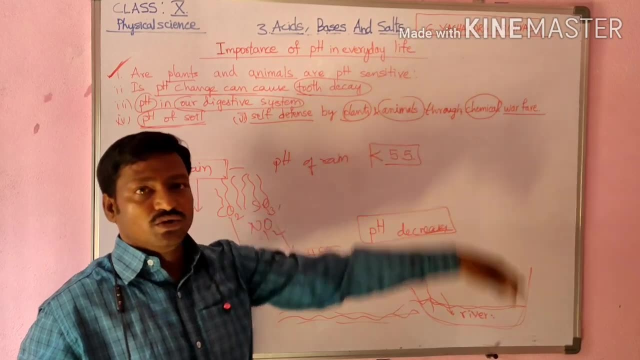 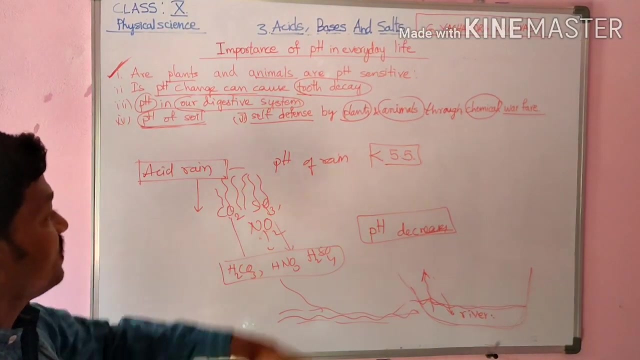 will affect the plants and animals so that's why we are saying that plants and animals are p-head sensitive so they can tolerate a narrow change in p-head if there is a drastic change 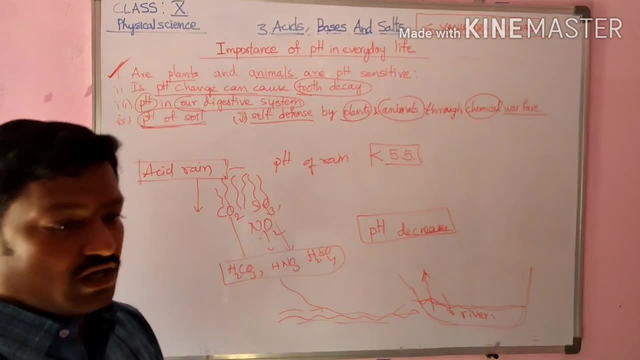 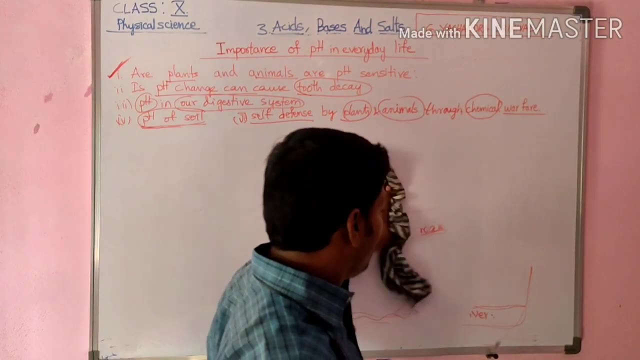 what happens the survival of the organisms becomes difficult right and next one is p-head change can cause a tooth decay so how this tooth decay occurs right so tooth decay tooth decay so tooth decay occurs when the ph of mouth when p-head of mouth is less than 5.5 where the ph of the mouth is 5.5 dreaded causes the so how this tooth decay 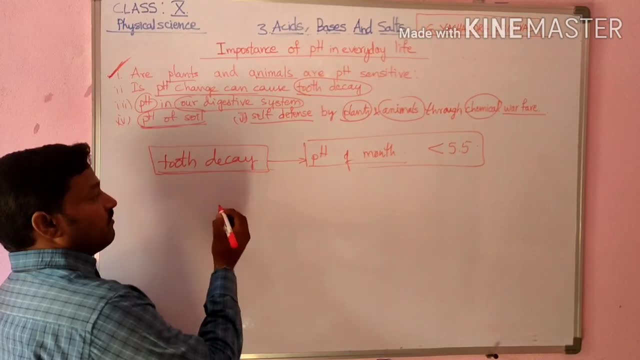 occurs so here when we eat the food when we are eating the food the food and the part thighs the teeth decay comes out diseases and dental will get deposited in between the teeth, in between the teeth. 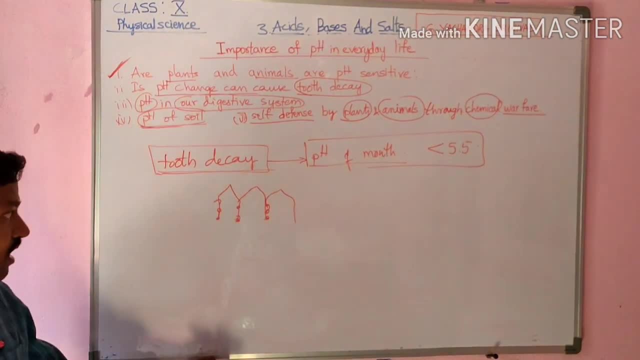 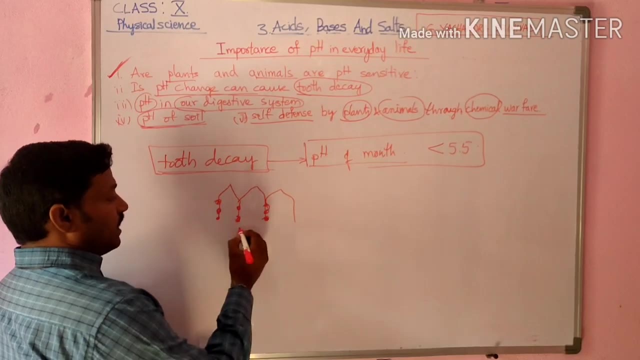 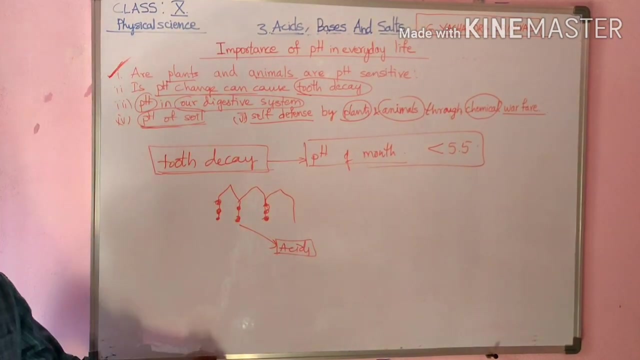 So, the bacteria present in the mouth, the bacteria present in the mouth degrades this carbohydrate, sugar particles into acids. These acids are produced by the degradation of food particles or sugar particles, right. 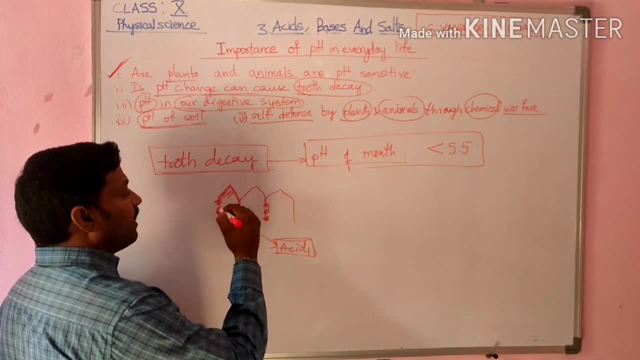 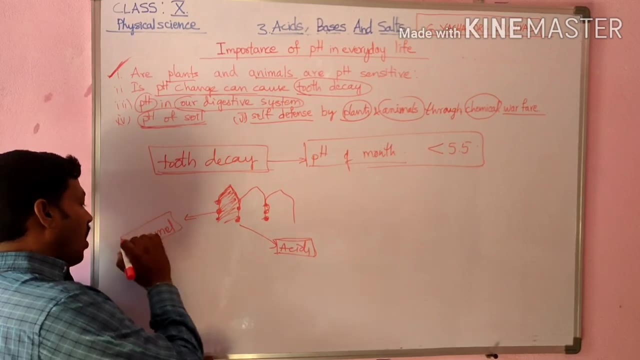 So, here this tooth is covered by a shiny enamel, shiny enamel, which is the hottest material in the body. 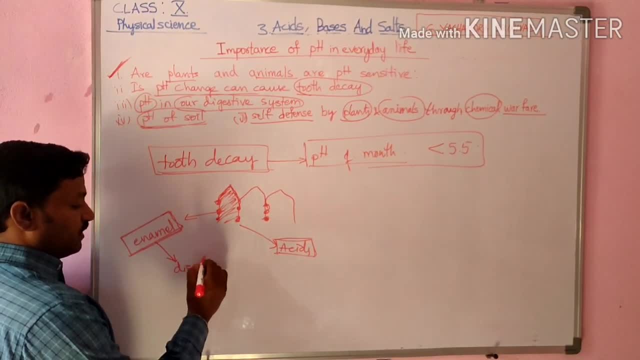 So, it does not dissolve in water, it does not dissolve in water, it does not dissolve in water. 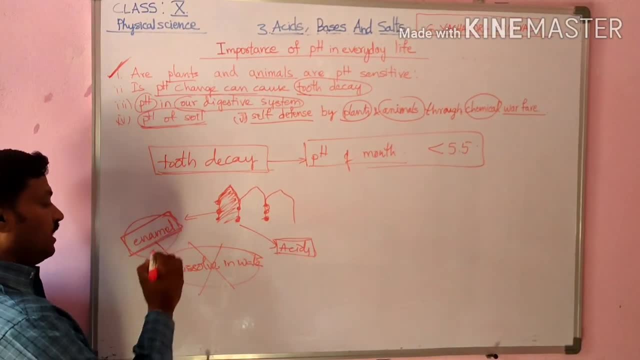 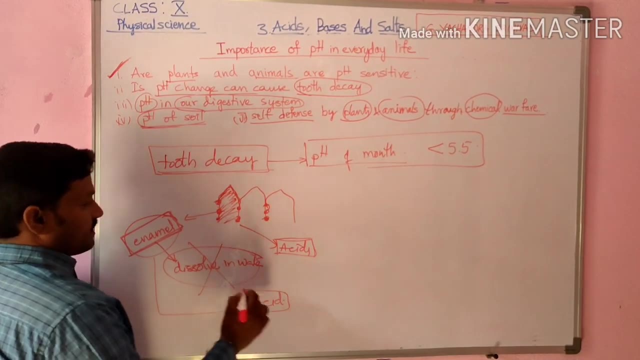 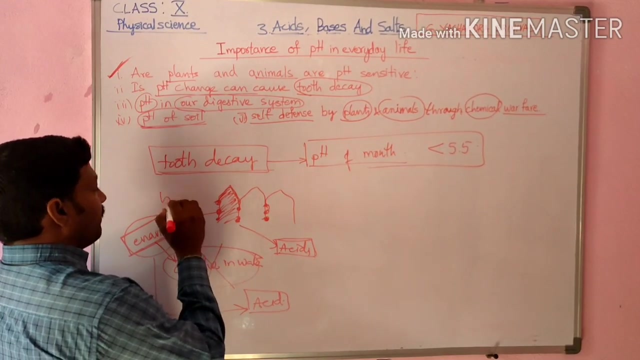 Whereas, whereas this enamel is corroded, damaged by acids, damaged by acids, right. When the food particles which are get deposited, they are degraded by the bacteria present 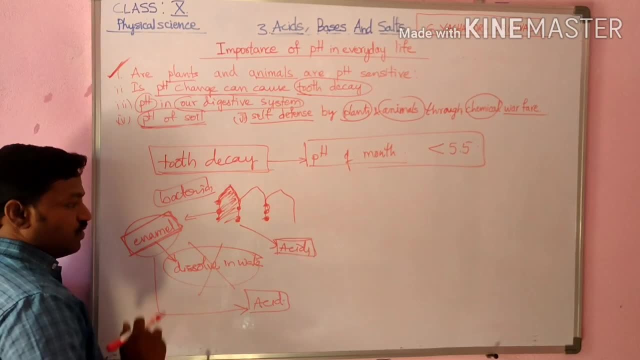 in the mouth causes the corrosion and that leads to tooth decay, tooth decay. 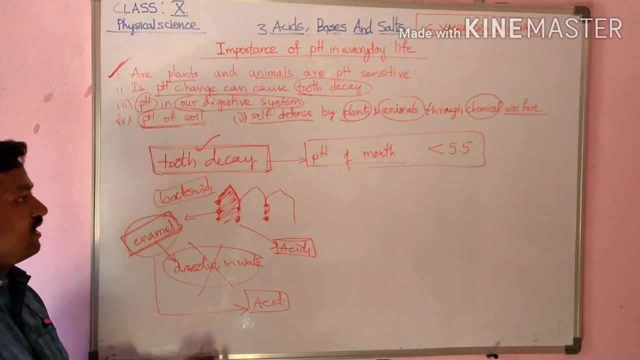 Right, so how to get rid of this tooth decay? 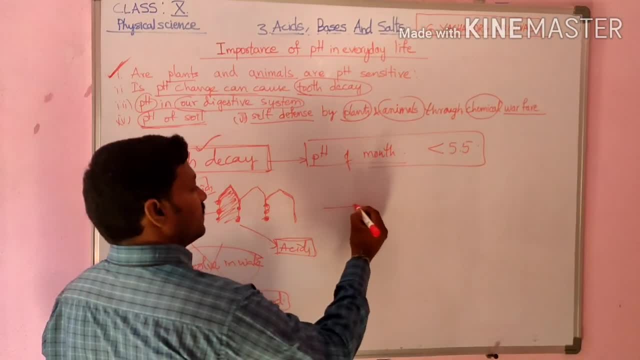 So, our mouth should be clean, right, clean with a paste, clean with a paste. What does the paste contain? 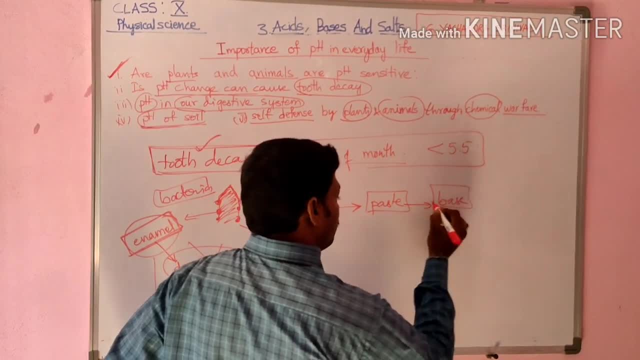 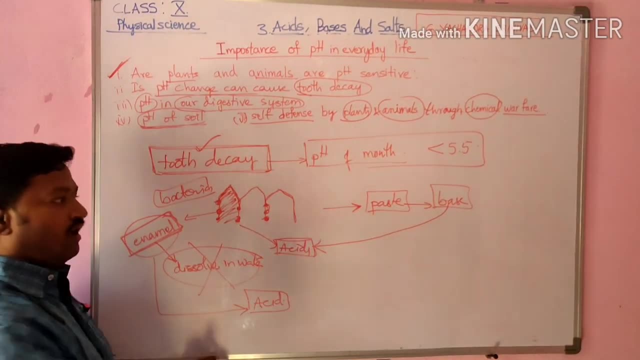 The paste contains a base, a paste contains, tooth paste contains paste. So, that paste will neutralize the acid. 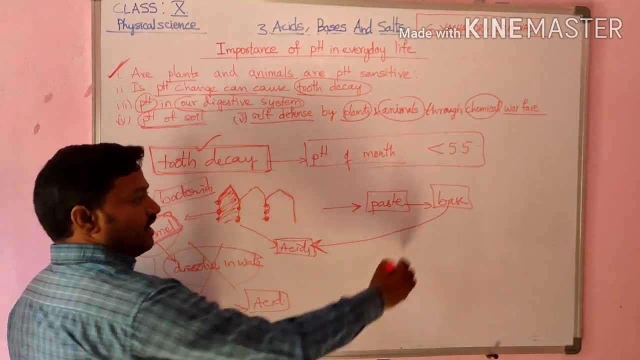 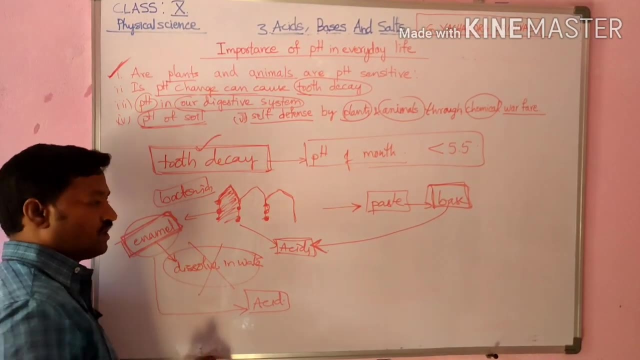 The acidic effect, the acidic effect is neutralized by the paste so that what happens this enamel will not be get corroded, understand, right. So, what does the tooth paste contains? It contains a base that neutralizes the acids in the mouth and prevents the tooth decay. 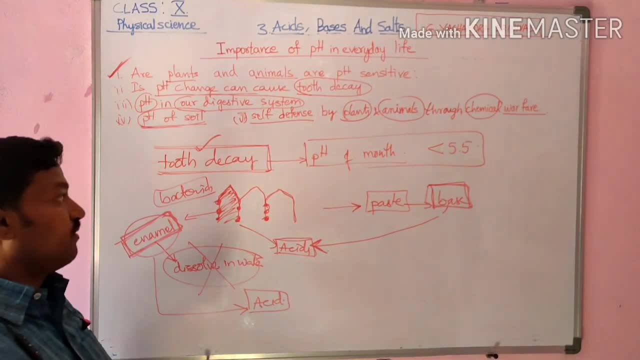 So, that's why it is said that we have to brush our teeth. We have to brush our teeth twice a day, twice a day, right. 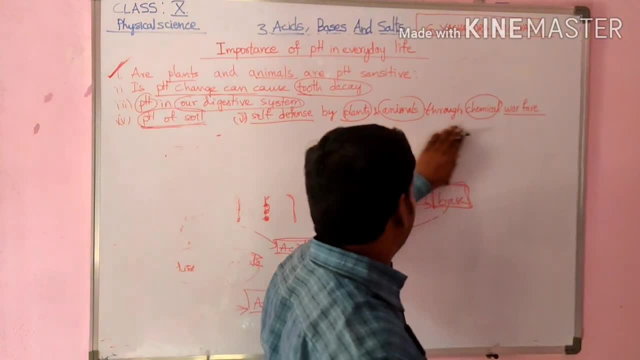 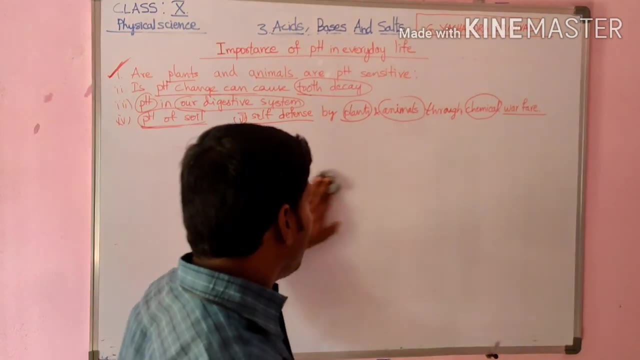 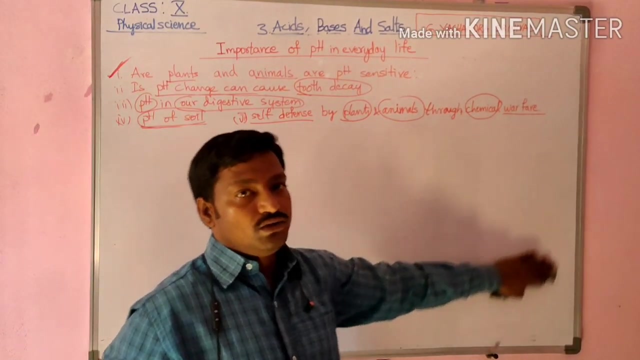 So, that is the reason, right. So, if the food particles are getting deposited, what happens? Those are degraded by the bacteria and that bacteria produces the base and that, sorry, produces acid, that acid will corrode the tooth and causes the tooth decay, right. 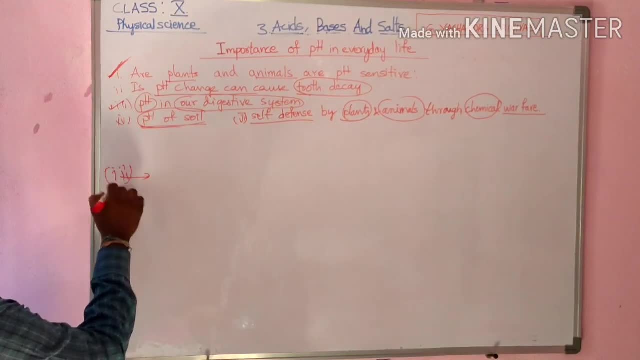 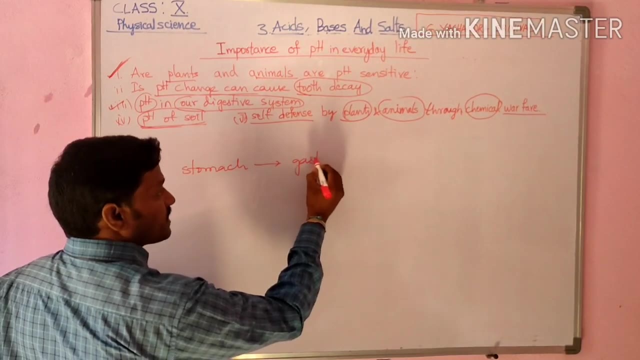 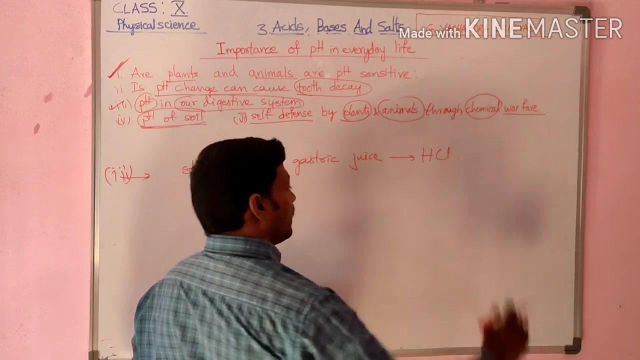 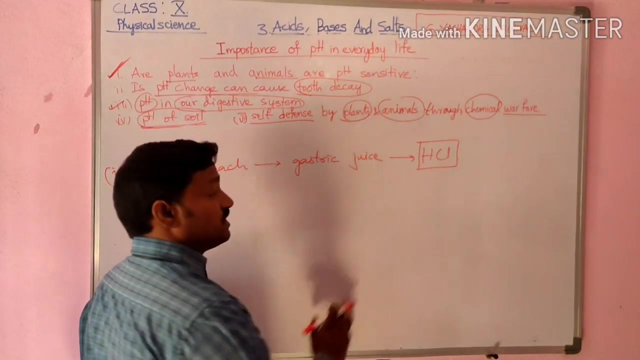 pH. pH in our digestive system. Already we have said, right, the stomach, stomach produces gastric juice, gastric juice, which contains hydrochloric acid and a digestive enzyme that is called pepsinogen, right, HCL, which is harmful. 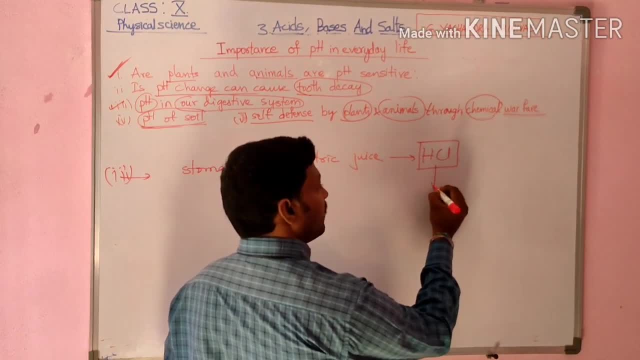 But in the stomach, this HCL helps in the digestion. Helps in digestion. 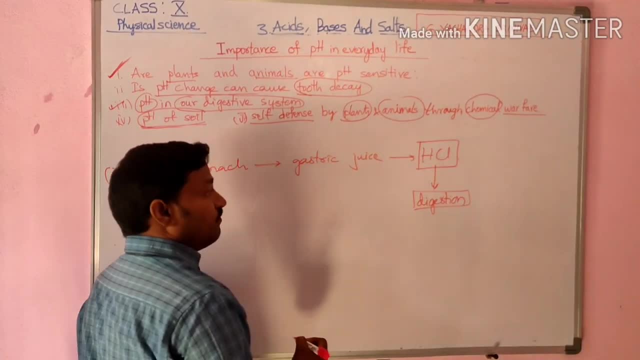 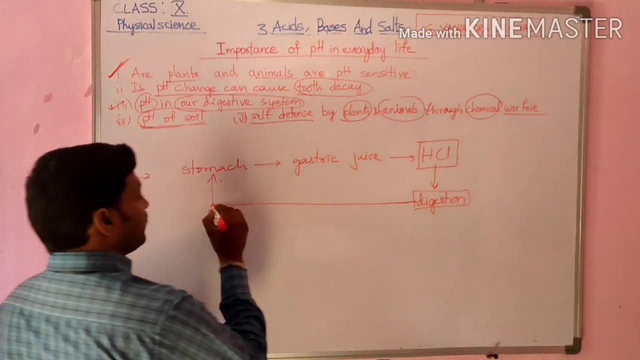 Helps in digestion without harming the stomach, without harming the stomach, right. 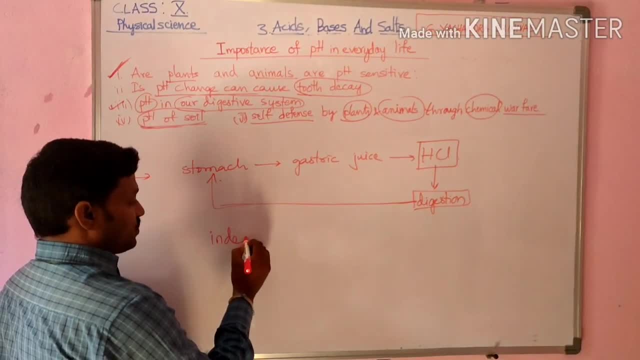 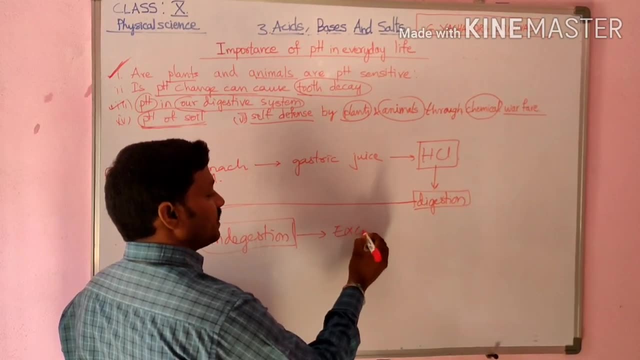 So, here, during indigestion, during indigestion, what happens? Excess of acid produces. Excess of acid produces in the stomach. And that excess of acid will cause the pain and irritation in the stomach. That causes pain and irritation in the stomach. And that pain and irritation is caused by excess of production of acid due to indigestion, is known as acidity. What is acidity? 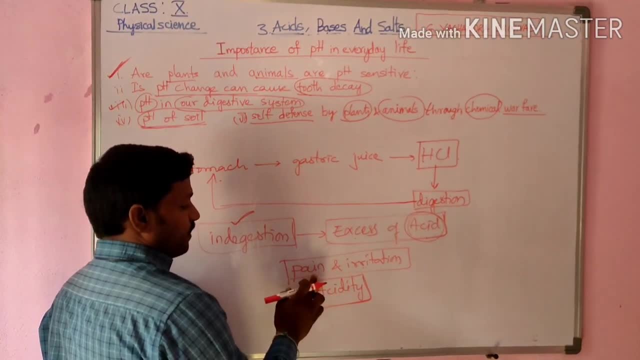 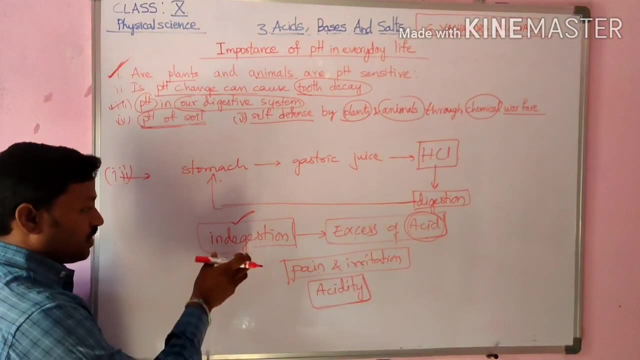 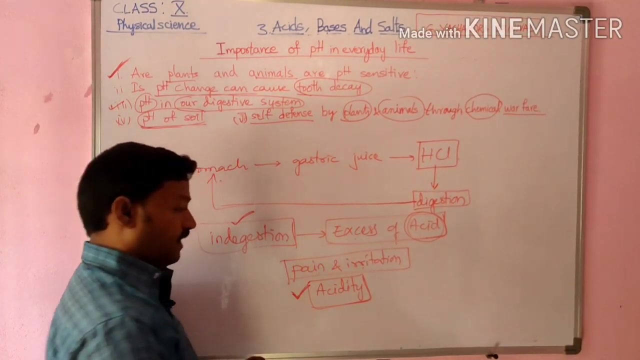 It is the pain and irritation in the stomach due to excess production of acid. That is because of indigestion. That is known as acidity. To get relief from acidity, we have to use a base. 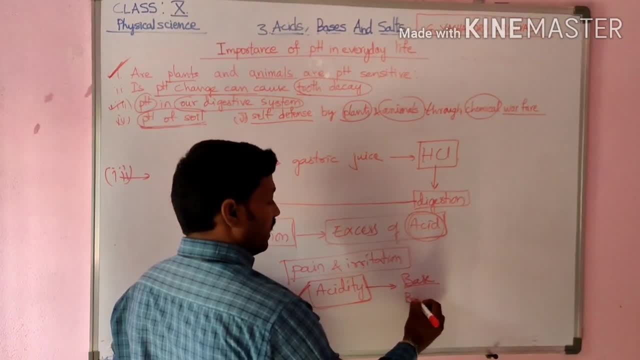 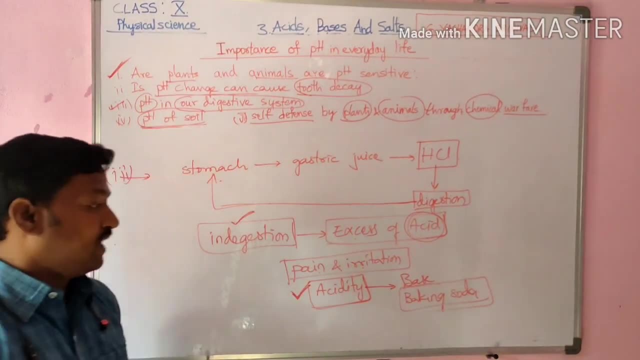 So, just like in our, in our houses, we use baking paper. in soda which is the mild base mild base baking soda is taken and that is dissolved in water and 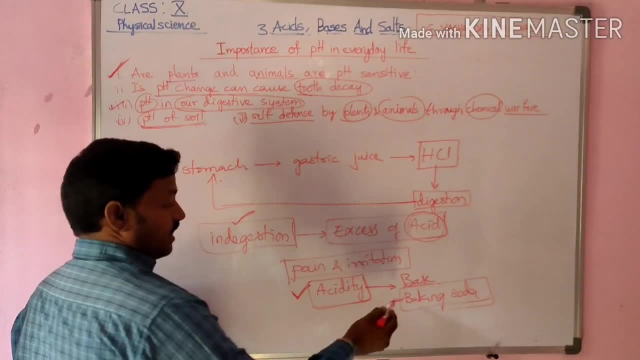 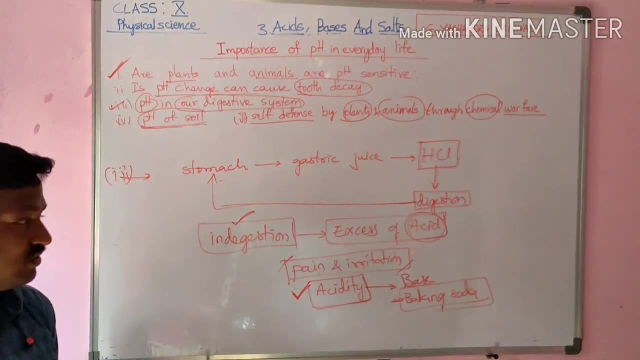 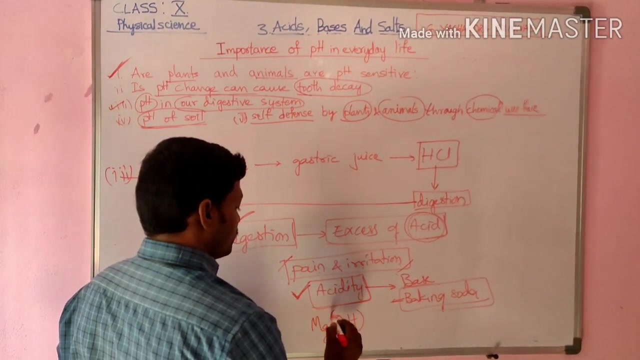 that water has is taken and that day it neutralizes the acid and release from pain and irritation that is neutralizes the acid and one more thing also we use that is called magnesium hydroxide 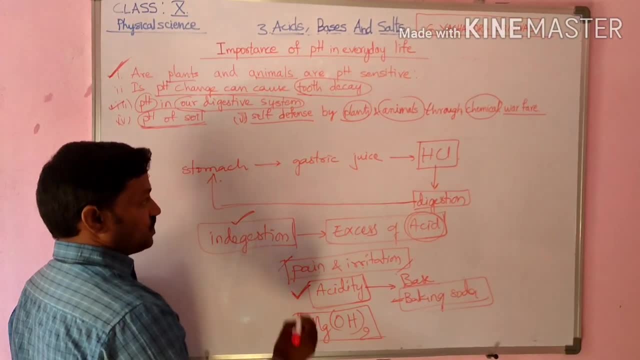 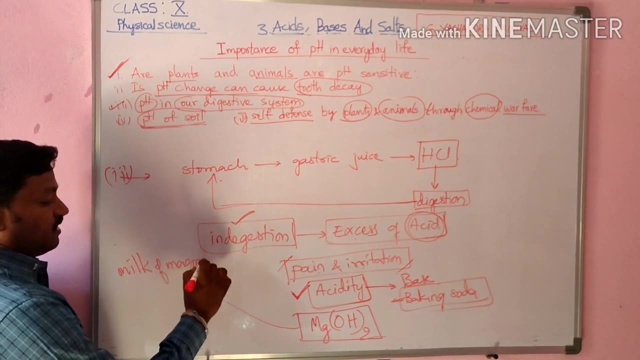 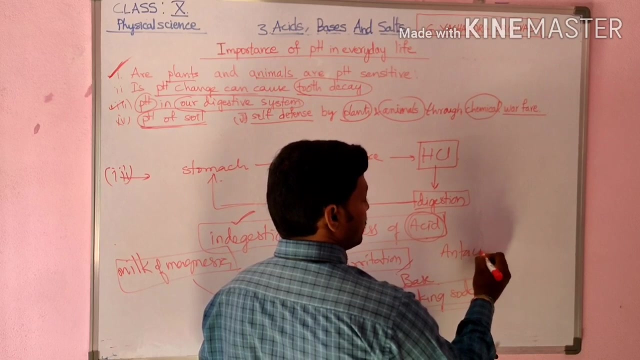 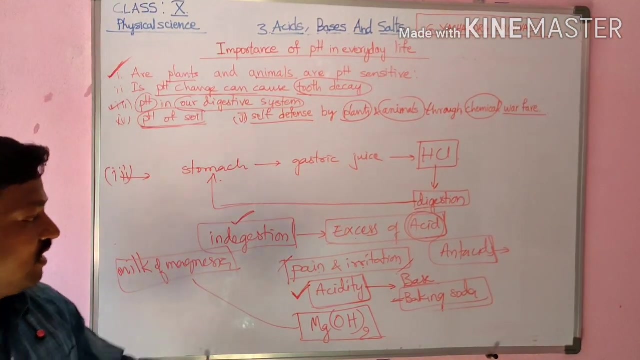 which is known as milk of magnesia which is known as milk of magnesia milk of magnesia ok so we use the tablets what are the tablets called antacid so what are those antacids contains a base which neutralizes the acidity 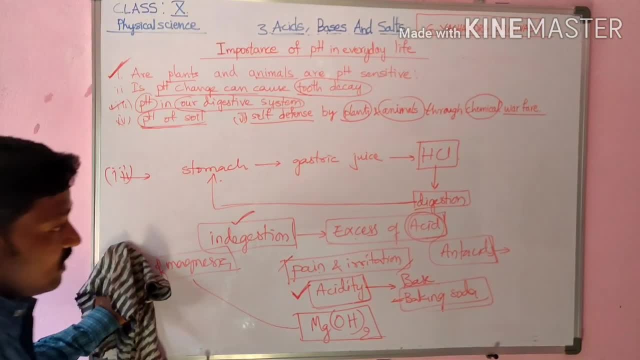 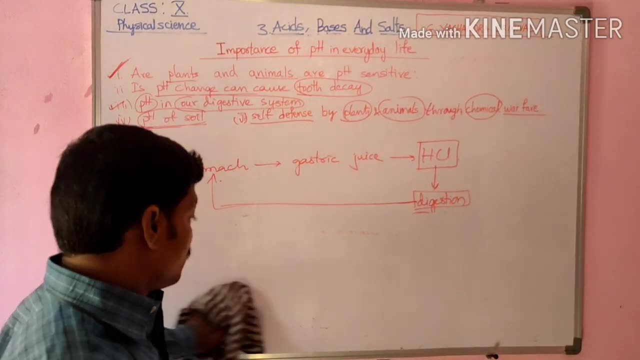 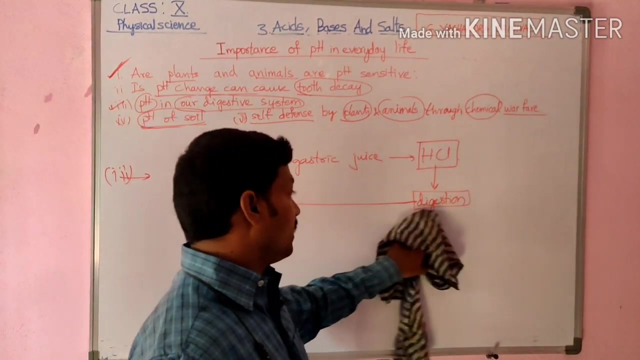 so generally in the market in the medical shop we will see what are those digene or you will see eno eno packets sachets out there right so those will help in neutralizing the acidity in the stomach and what does that antacid contains what does antacid contains 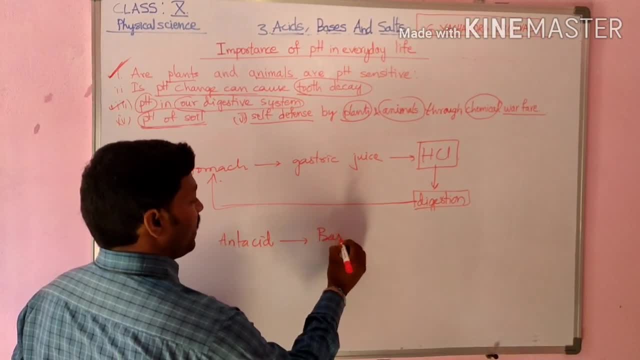 antacid contains a base that neutralizes the acidity in the stomach 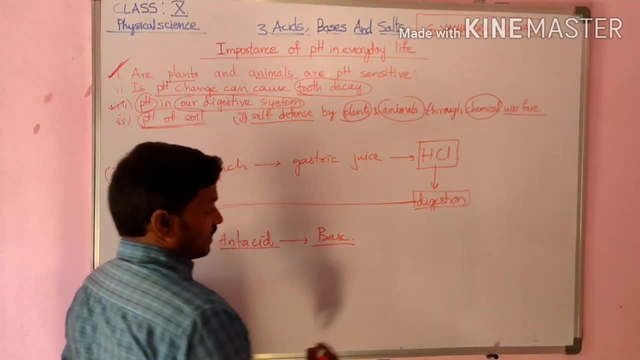 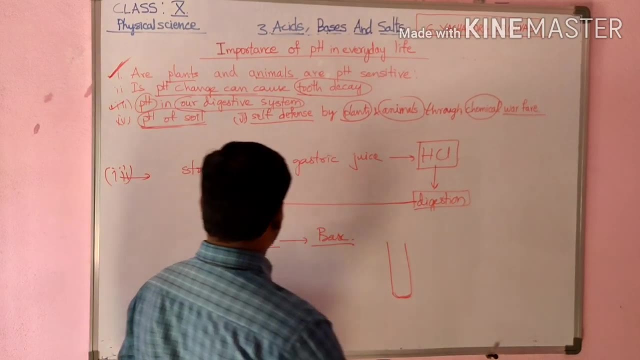 right so let us see the how this antacid acts right so take a tested tube ok a tested tube 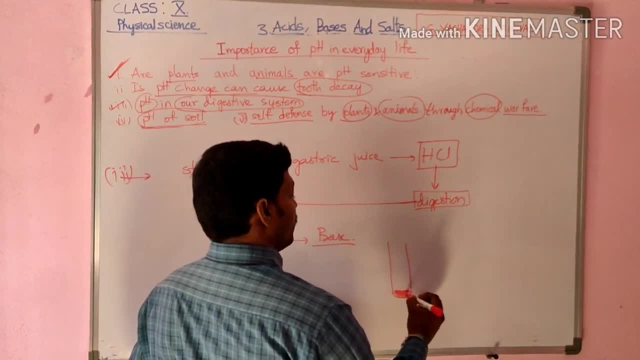 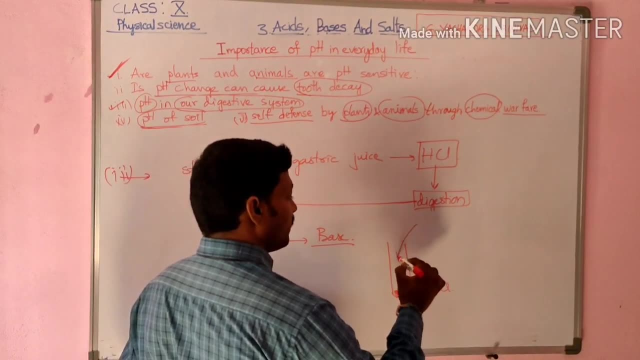 and take some amount of diureth hydrochloric acid diureth hydrochloric acid and do this act 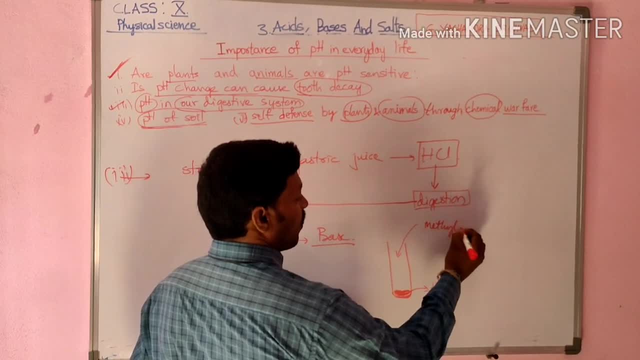 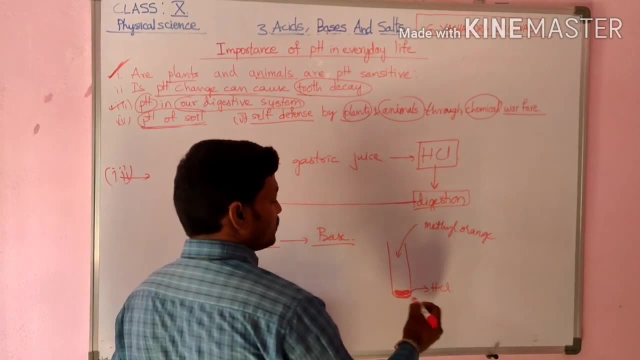 one or two drops of methyl orange methyl orange is added so because of adding this methyl orange to the acid 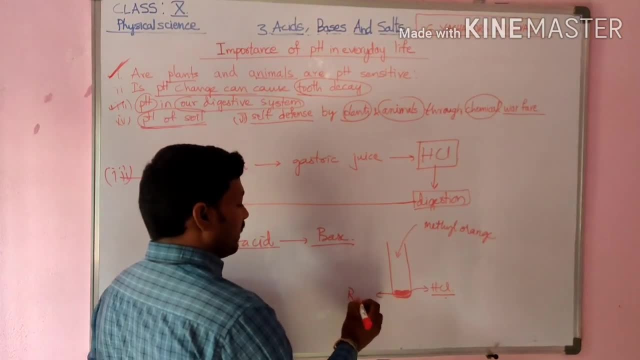 then the colorless hydrochloric acid turns to red color 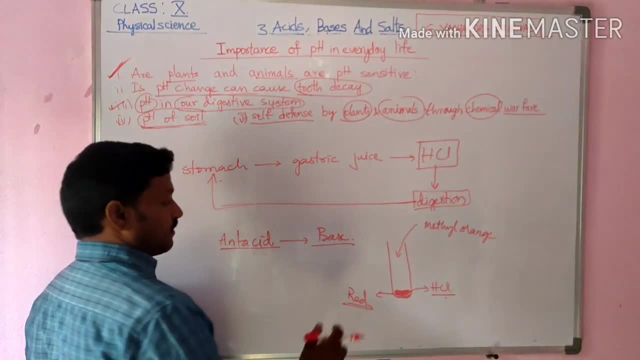 the acid turns to red color ok 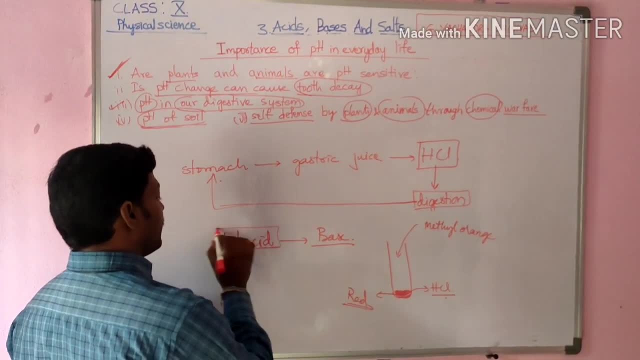 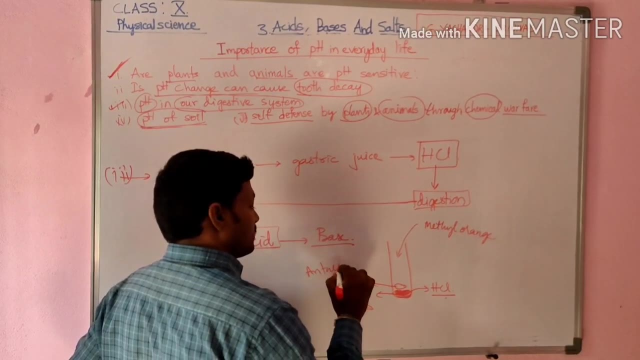 so now to this acid we have to add an antacid tablet antacid tablet antacid tablet is added to this acid 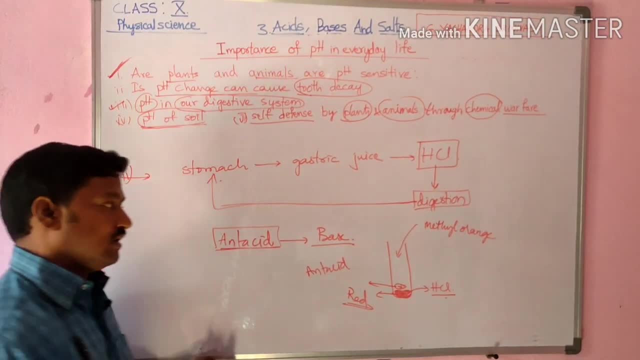 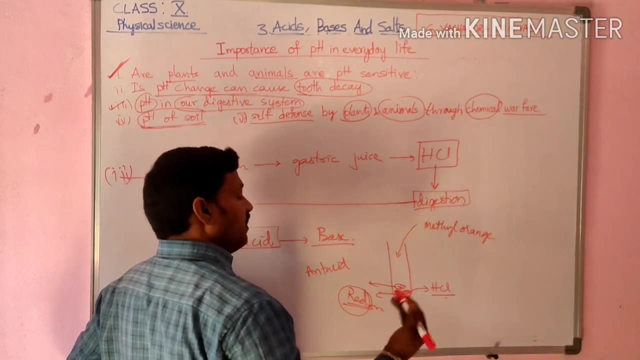 then we will see the change in color right so the methyl orange changes to red color right so the red color slowly fades up 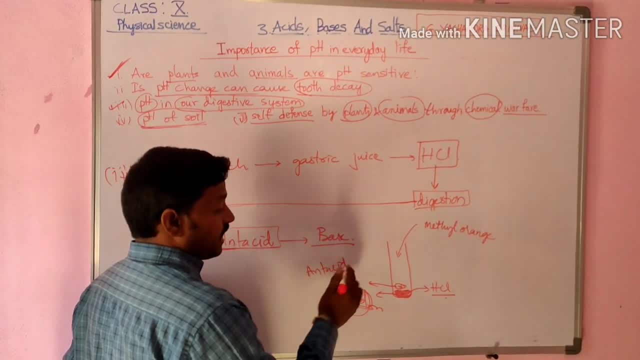 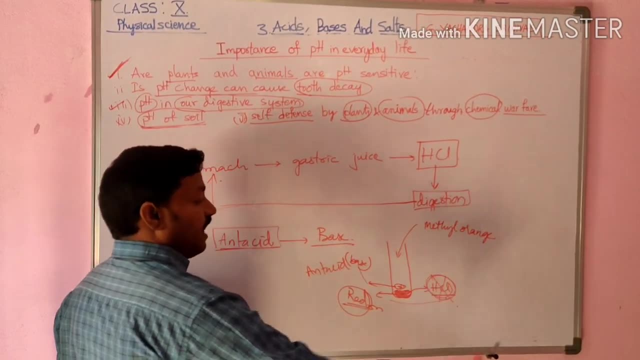 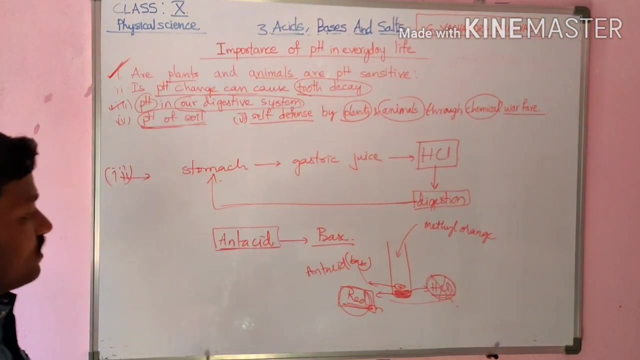 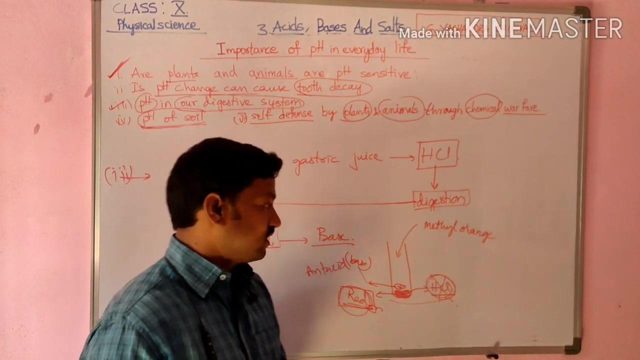 why because this antacid contains a base and that base will react with the acid and nullifies this acidic character thereby what happens the red color slowly disappears so from this we can understand that the base reacts with acid and giving rise to neutral that is salt plus water that is known as neutralization reaction 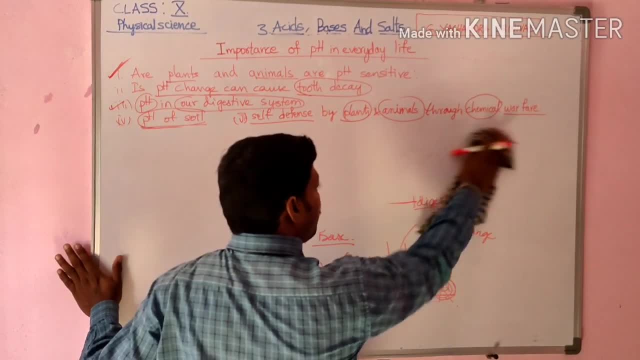 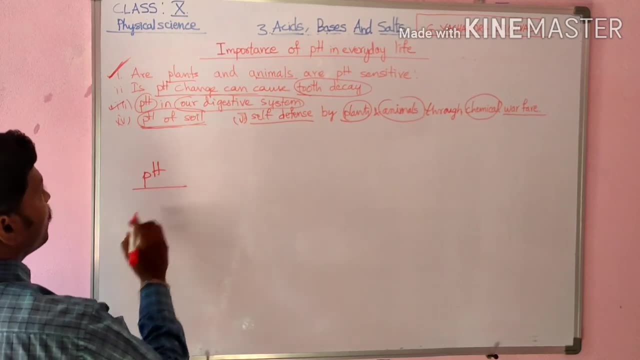 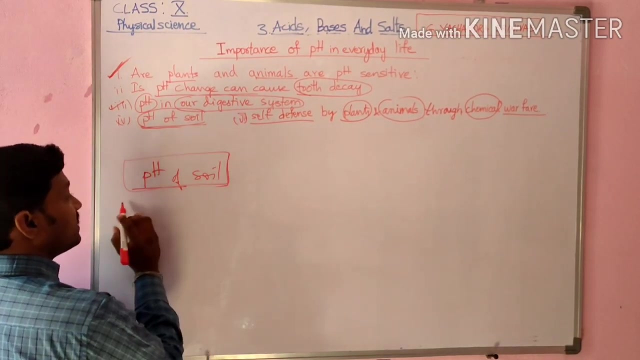 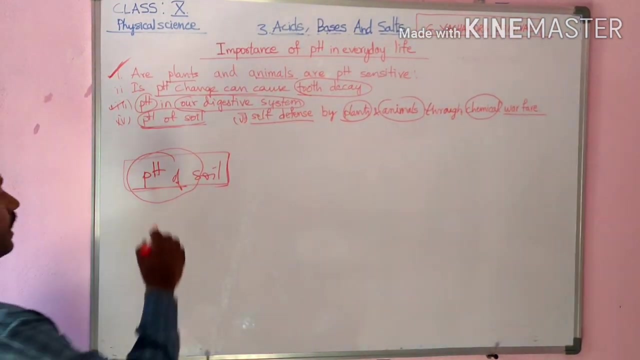 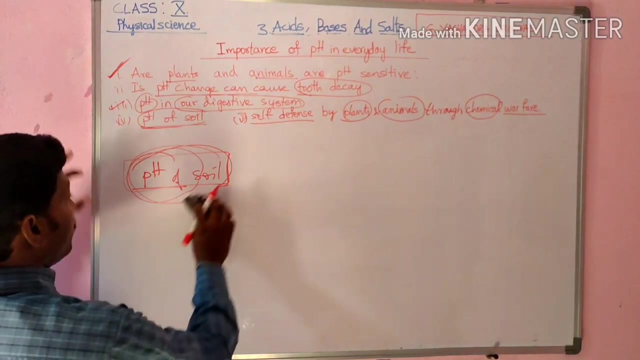 now coming to pH of soil so plants will grow at a particular pH plants for the healthy growth of plant for healthy growth of plants the plants need a particular pH of the soil particular pH of the soil at a particular pH of the soil only the particular plants can grow very well so if the pH changes then what happens 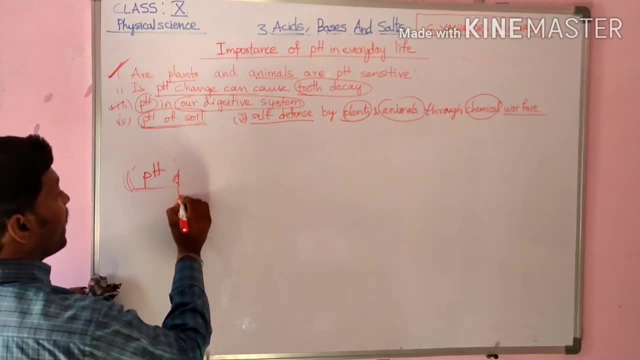 that will affect the growth of the plants growth of the plants 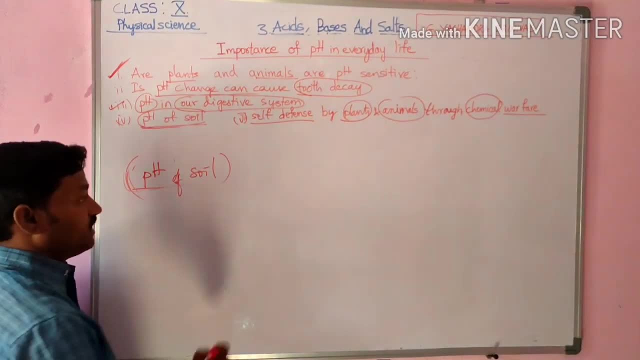 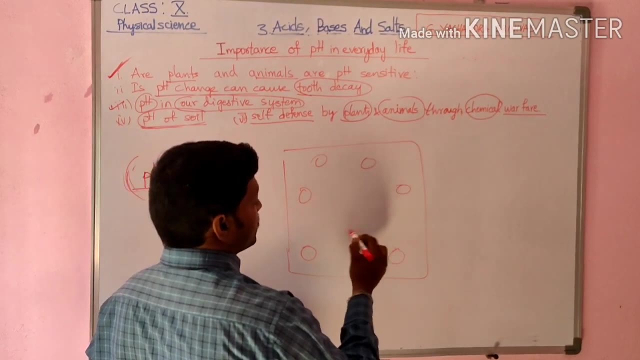 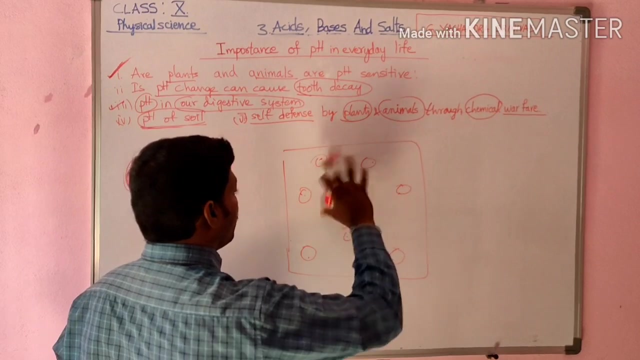 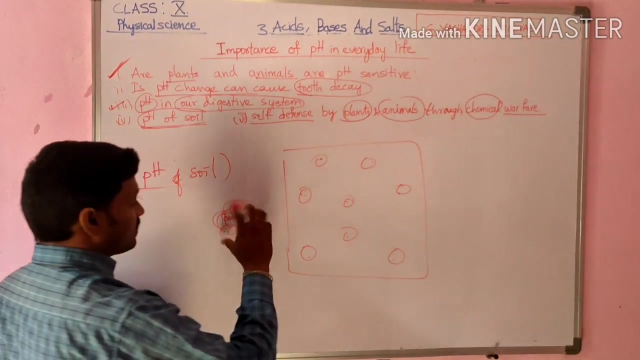 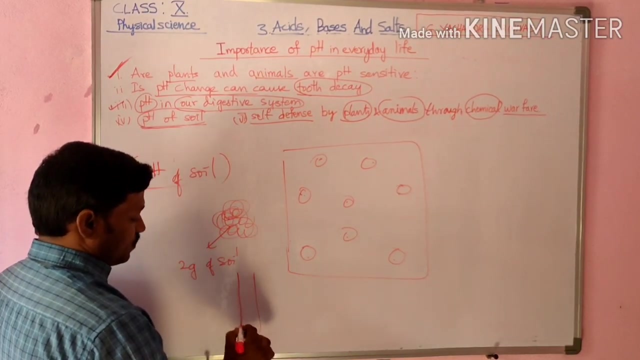 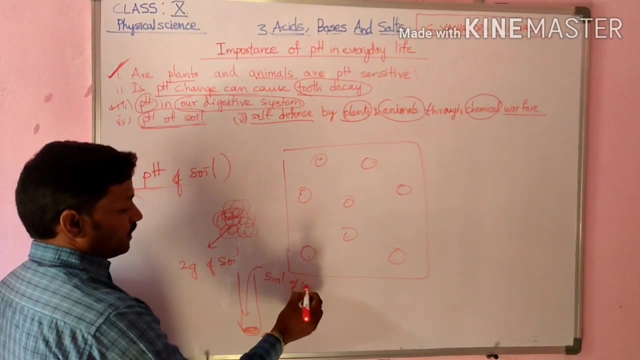 so how to know the pH of the soil first is right let us take this is a field and we have to collect the soil at a different places in the field we have to collect the soil from different places in the field and mix them all mix them all right so what have collected those samples are get mixed and you take 2 grams of soil in a test tube 2 grams of soil in a test tube and to this add 5 ml of water 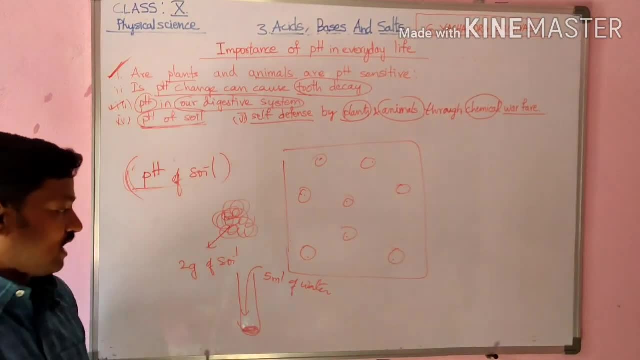 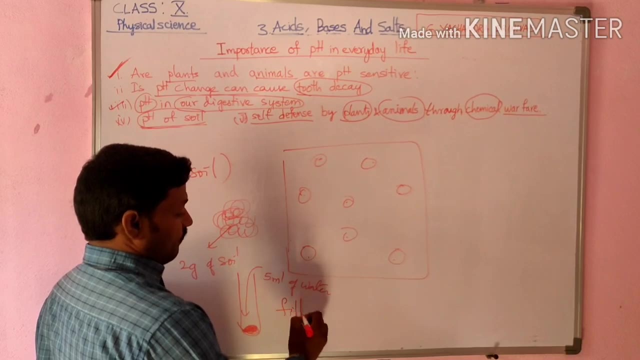 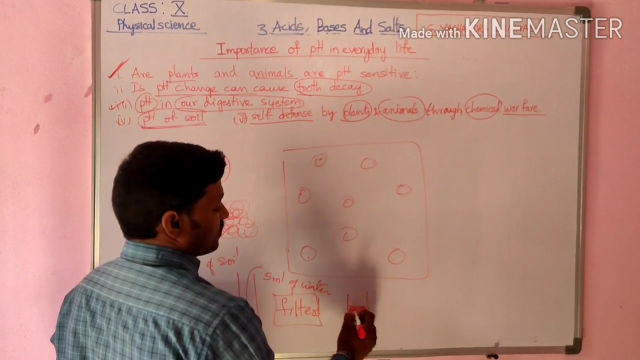 5 ml of water and stir it well and after that you have to filter this solution filter this solution and you will get a clear liquid solution 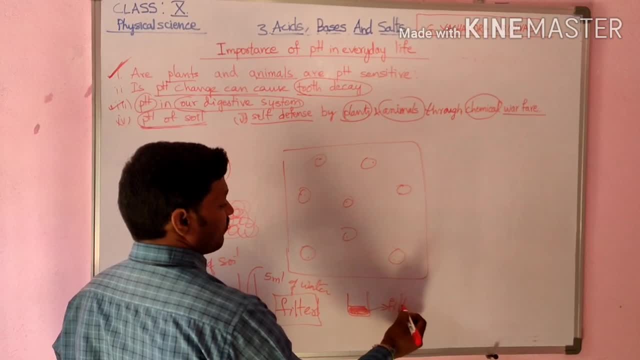 that is known as filterate 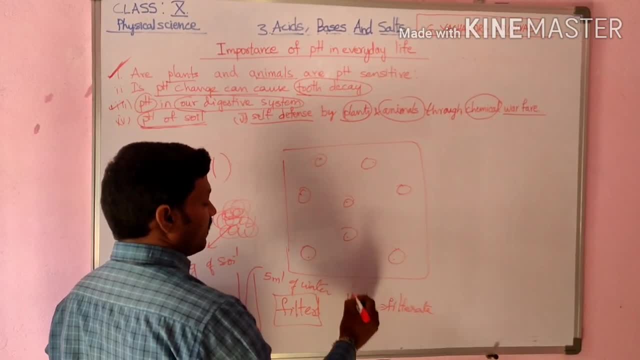 filterate right now test this filterate with the help of 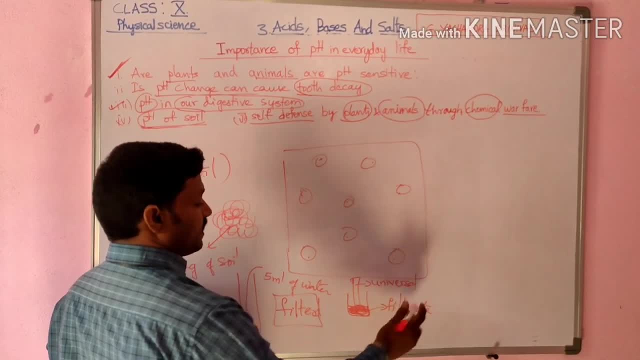 universal indicator test the solution with universal indicator 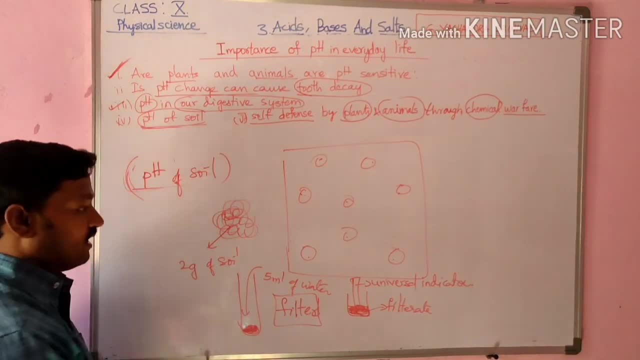 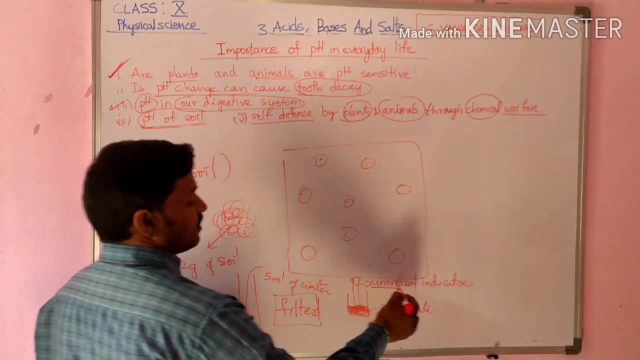 right so the change in colour will indicate or it will give the particular pH of the soil ok so by using the universal indicator 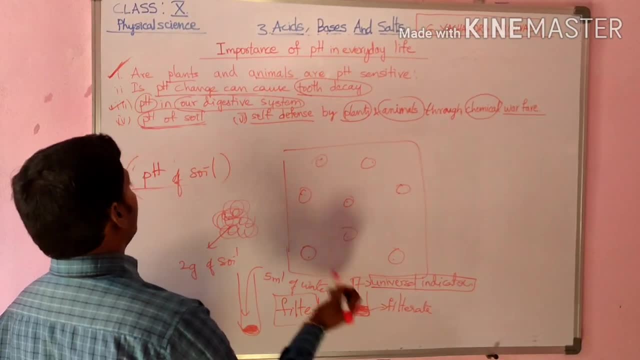 we will know the nature of the soil ok this is how we will identify the pH of the soil 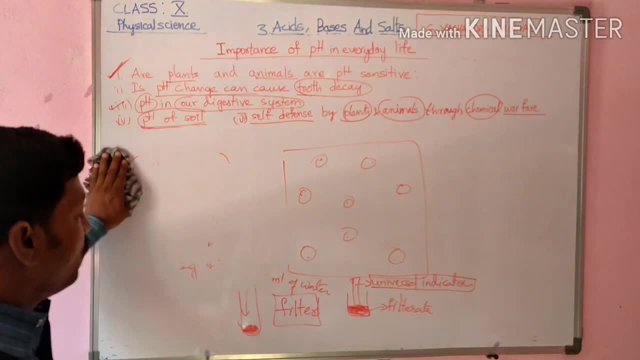 and next one self-defense by plants and animals through warfare 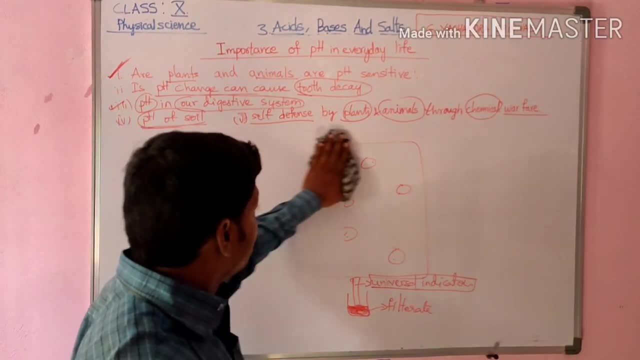 right so these plants and animals will get protected they are protected from the enemies right through those chemicals 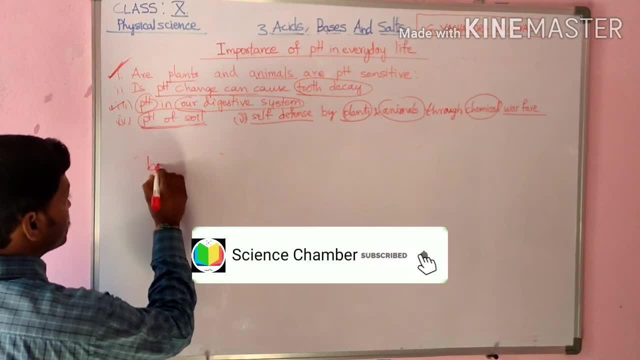 right how for example if you are taking bees honey bees 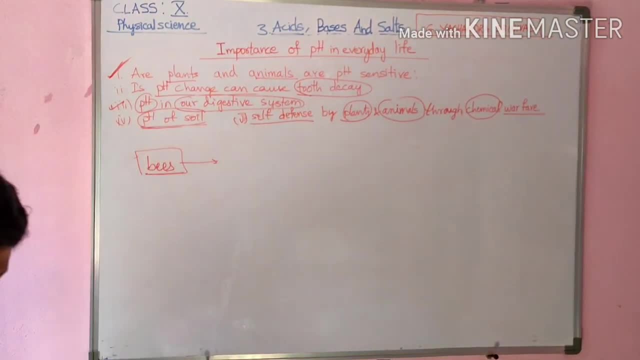 right so when they are when they are stung us 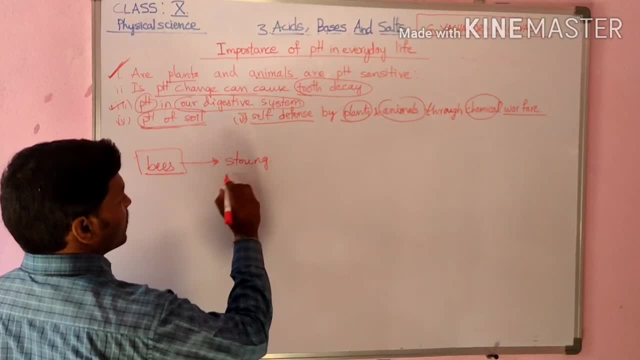 when they are stung us stung us then what happens they will inject acid 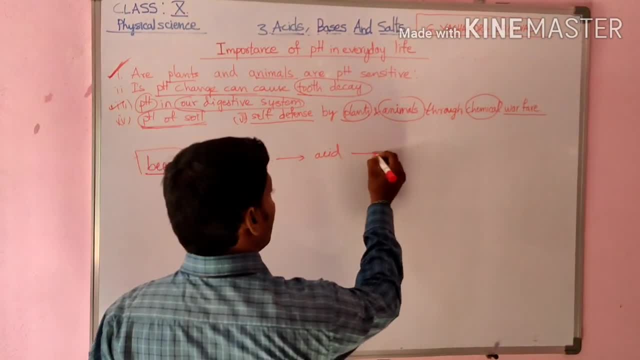 they will inject acid what is that acid methanoic acid 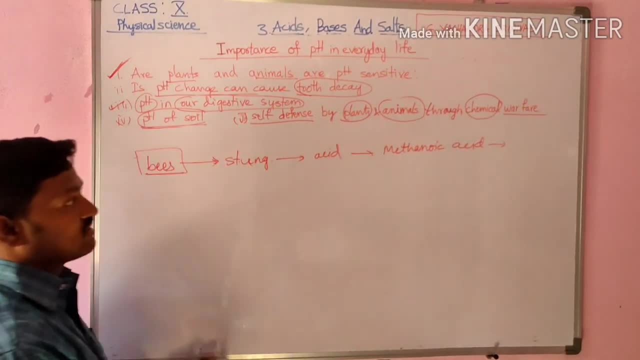 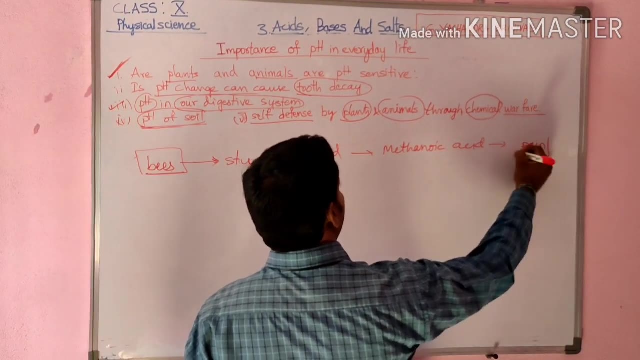 methanoic acid they will inject methanoic acid so this acid causes the pain or the burning sensation that causes pain or burning sensation 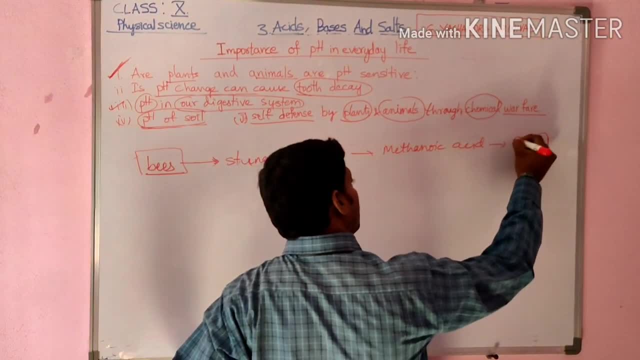 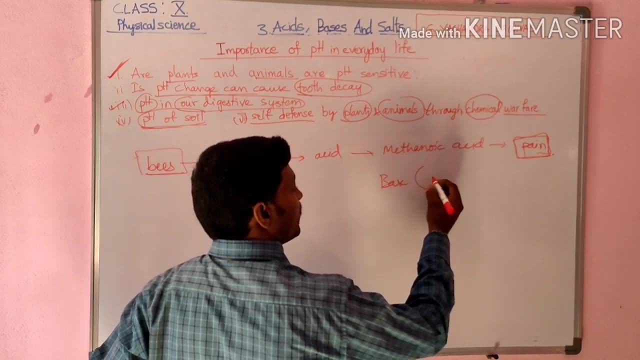 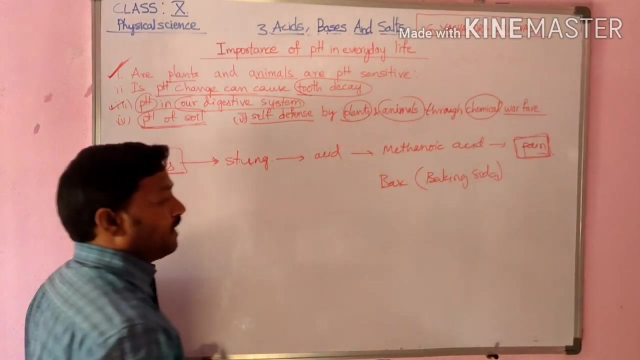 right so this pain can be relieved by wrapping that affected part with a base usually we use we can use baking soda baking soda which is a mild base 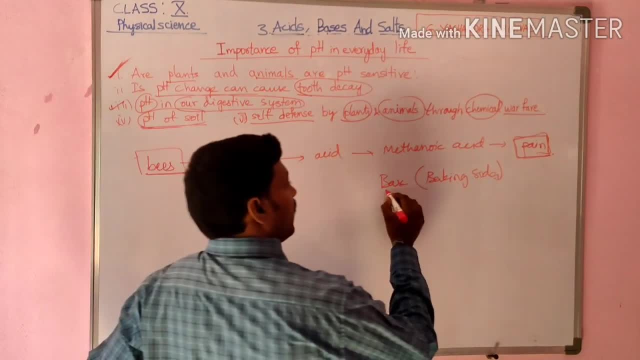 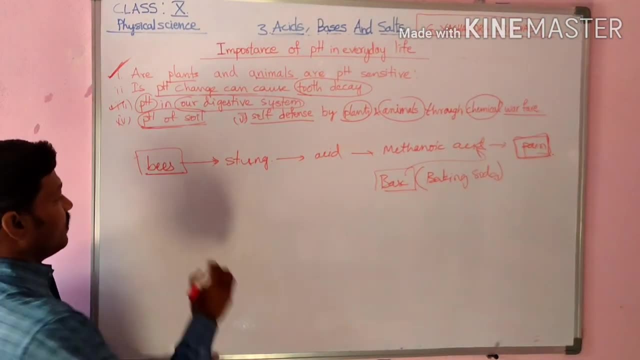 that affected part is wrapped with a base then what happens this base will neutralize the acid right and ants also use that 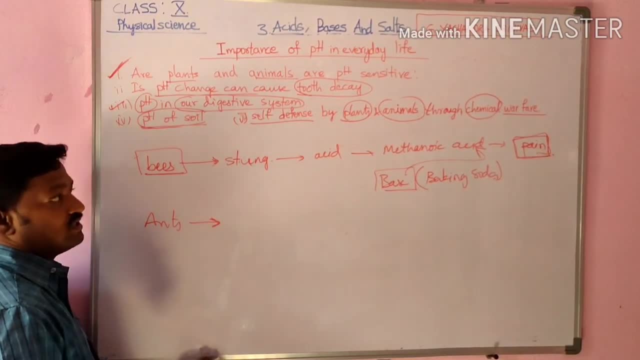 when they bite us they will also inject an acid called 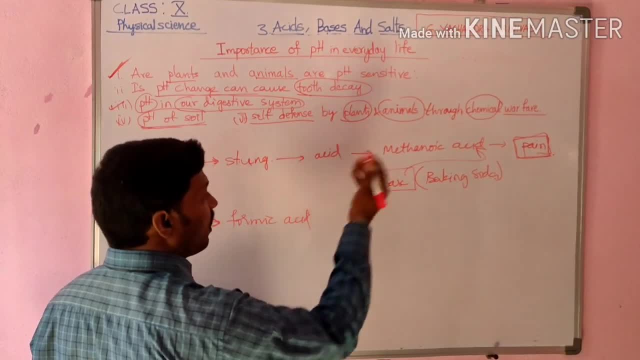 formic acid formic acid or you can also call that methanoic acid 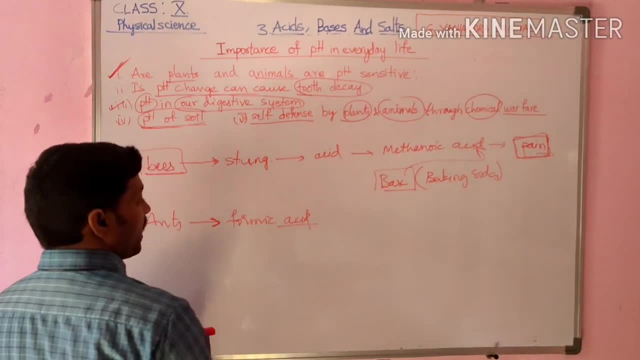 and you know that how to relieve this pain right by using the base so the base nullifies the acids 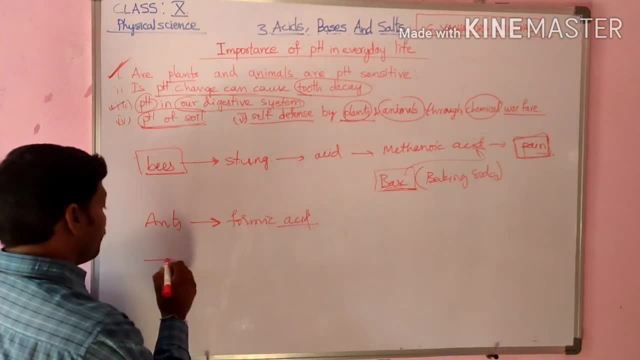 in the same way how plants for example stinging hays 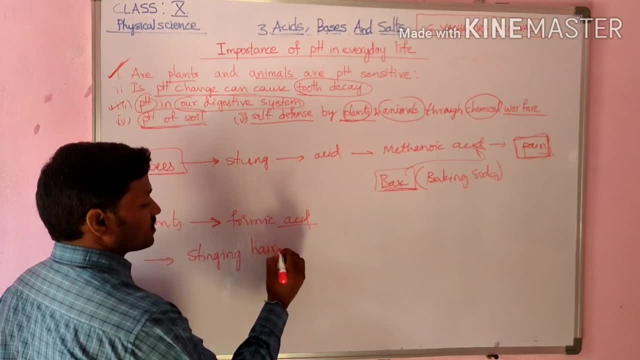 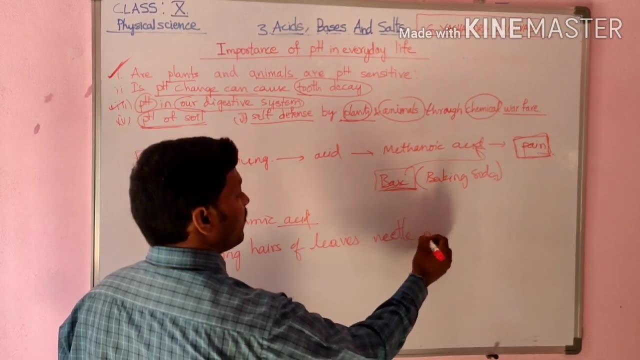 stinging hays of leaves of nettle plant which plant nettle plant 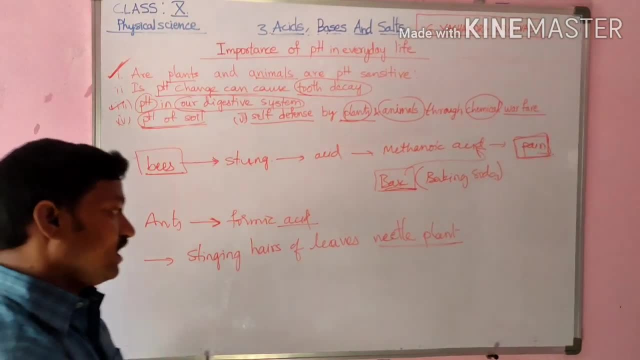 when it is stung us then what happens it also injects an acid called